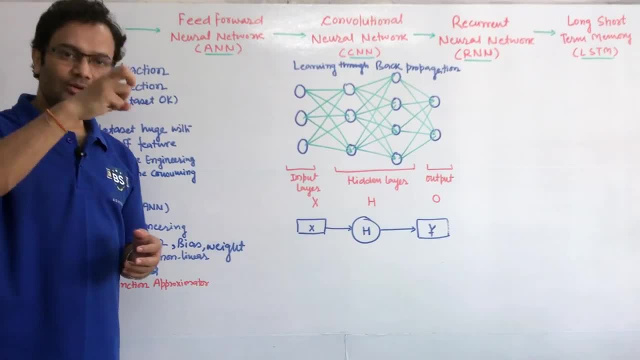 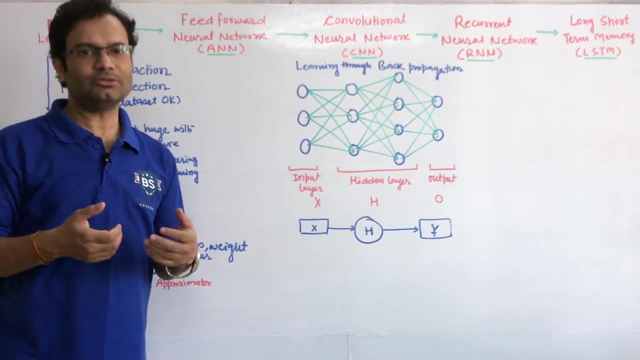 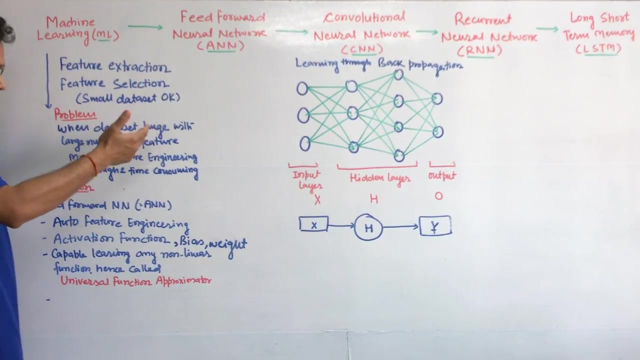 features. it is not easy to extract those features and select those features. We cannot do that manually right. it is very time consuming and not possible at all also. So those kinds of things, you cannot do that. So then what is the solution for those use case? 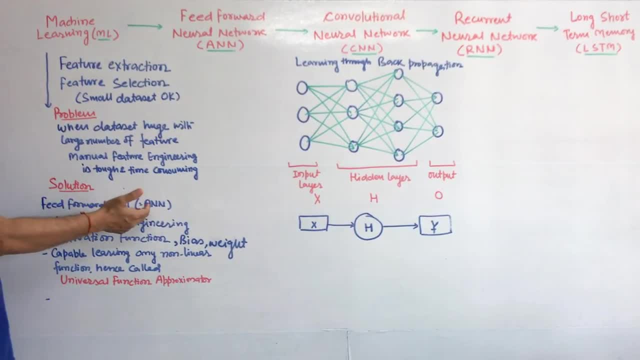 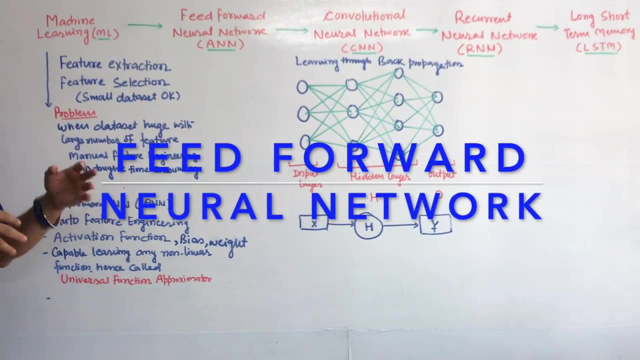 So solution is that ANN, like the feed forward network. this is the solution right Here. we do the auto, auto, auto feature engineering. So no need to do all those things- feature extraction and selections- that we do themselves using the algorithm. 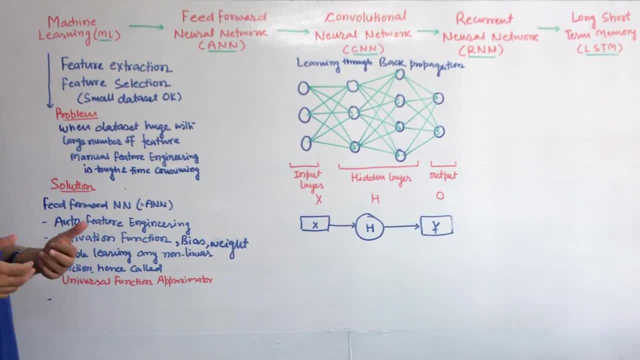 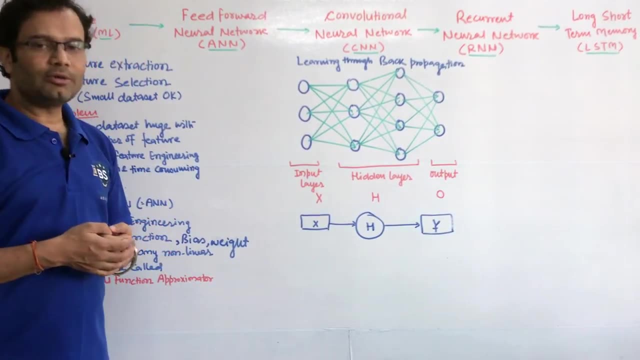 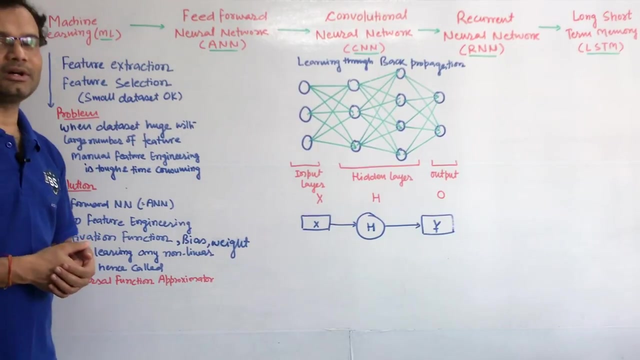 So that is called the auto feature engineering And we have the concept of the activation bias weight. all those concepts come in the feed forward neural network right And due to those concepts it is capable to running any non-linear function, even they. 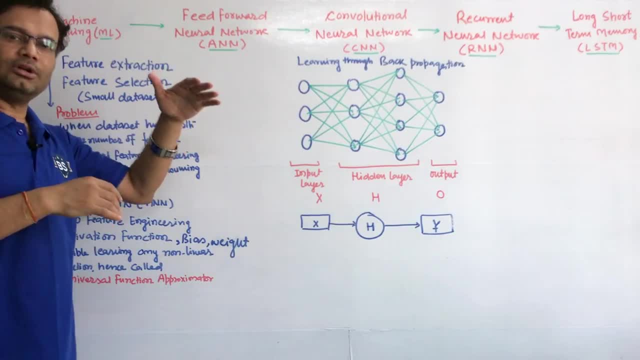 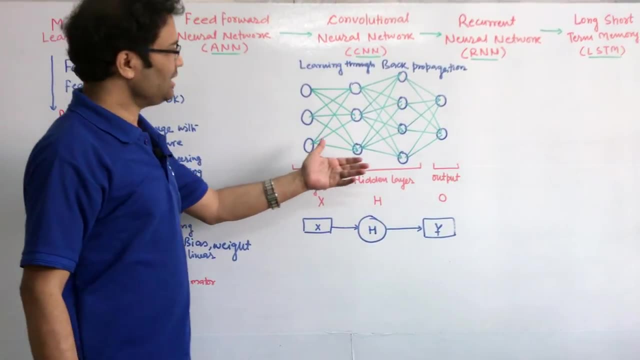 do not have the easy separable, even those functions. we can do that, And that is what is called the universal feature approximator, And this is the typical diagram for the ANN right. So this is the typical diagram for the ANN right. 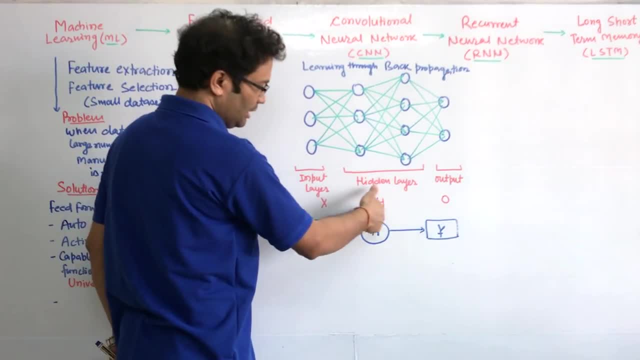 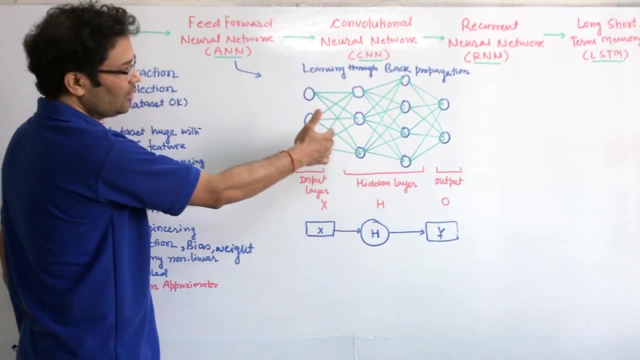 If you see in this diagram, we have the input layer, we have the, we have the hidden layer, we have the output layer And we can have the multiple hidden layer. depend upon the requirement And on the each neurons or the neuron unit. so what we used to do, we have the input. 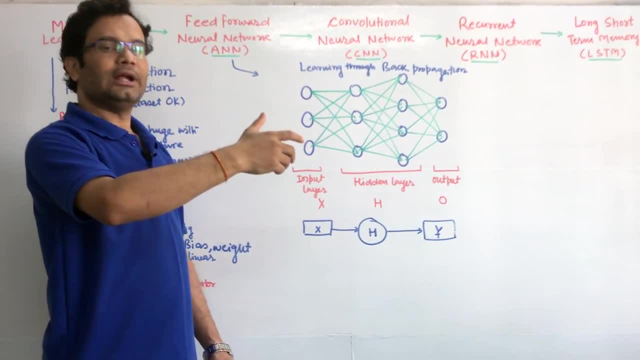 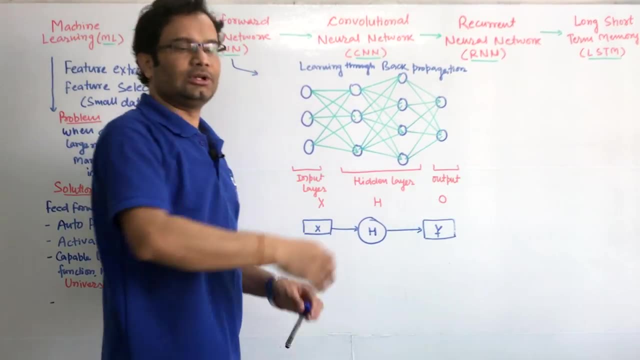 we have to weight, we multiply the input and weight and we add the bias, it go to the different activation function And finally you can get the output. And once you get the output, once you done the feed forward, propagation we have to do. 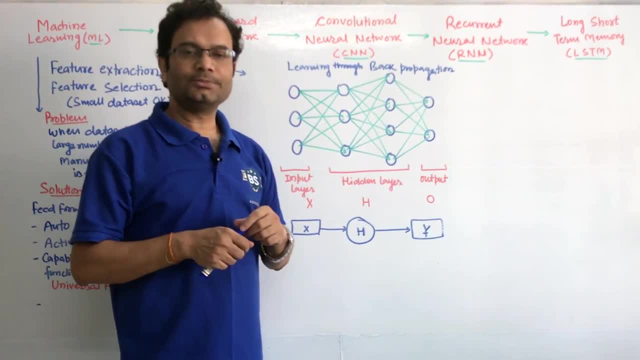 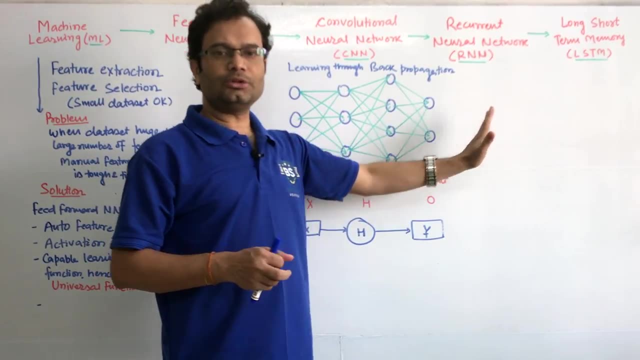 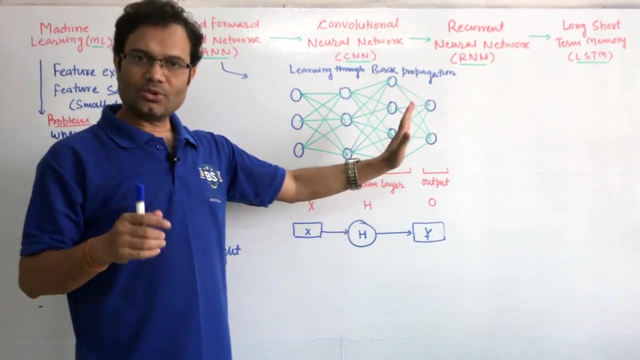 the back propagation, to modify the weight, to minimize the error. So what we used to do at this stage you will get the model output and we have already the our known actual output. We differentiate, make the square that is called the error. 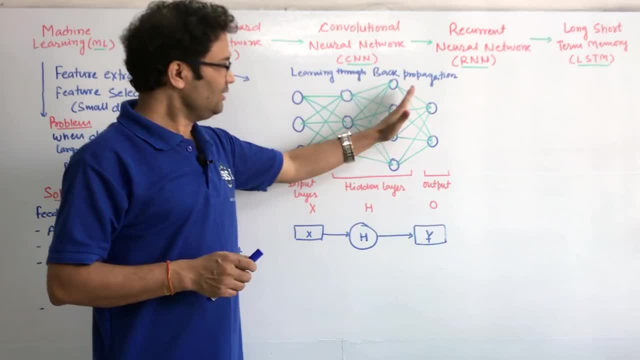 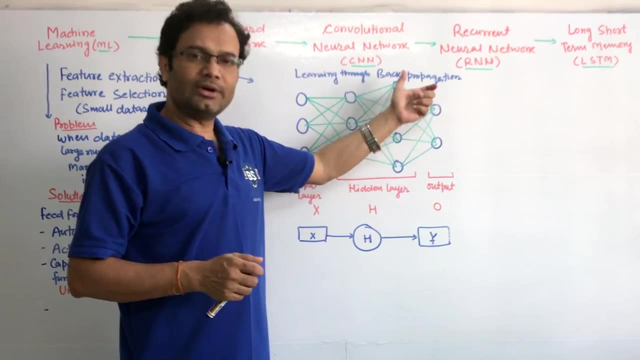 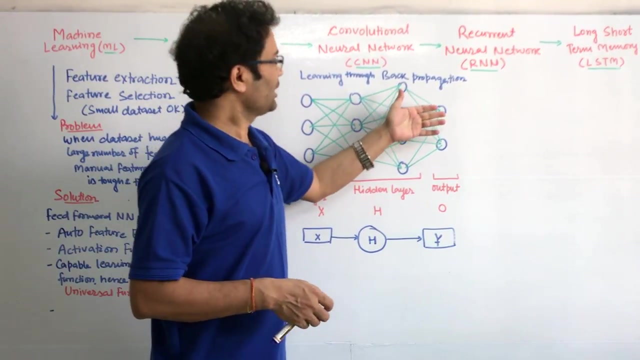 On those error, differentiate the error. We differentiate those error with the individual weights and once you get the difference of air, difference of the weight, we modified the weight and this is the way depend upon the EPOC. we can go the, we can go the multiple times for the back part, propagations and finally, 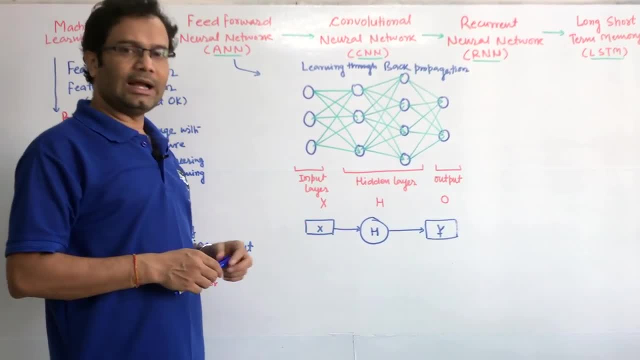 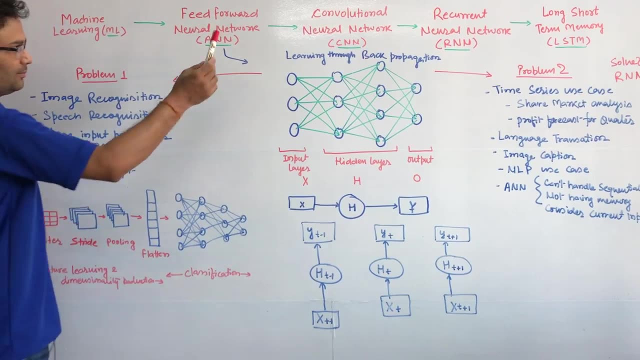 we can get the solution, But here also we have the some problems that not able to solve the CNN. So this is the problems. This is the ANN. Okay, We don't confuse with the CNN. This is the ANN diagram, right? 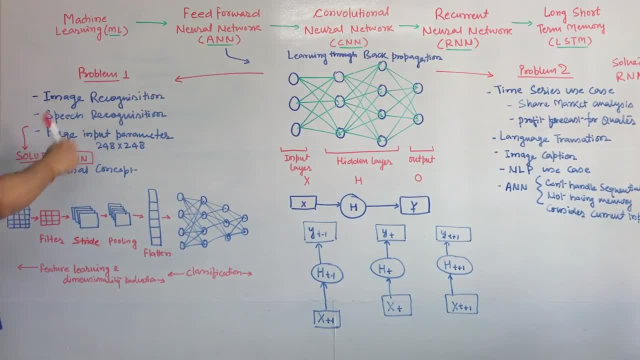 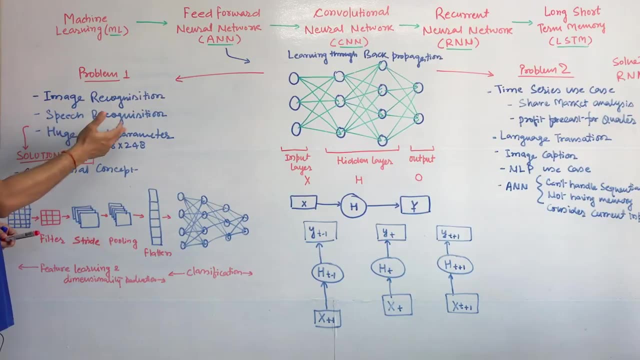 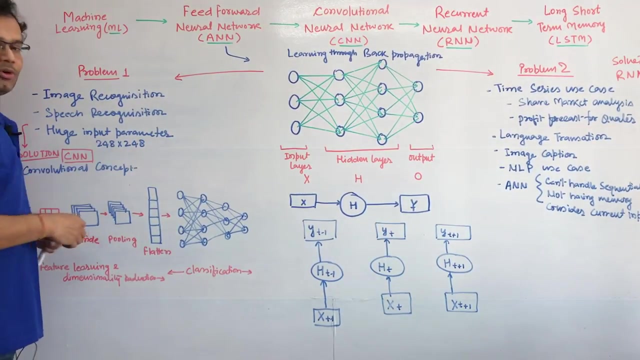 So now, what is the problem of the ANN? First problem is that if you want to classify the some image, or if you want to recognize the image or the speech recognition, we can't do it here. The reason behind that: if you take any good image, if size is the 240 by 240, if you multiply, 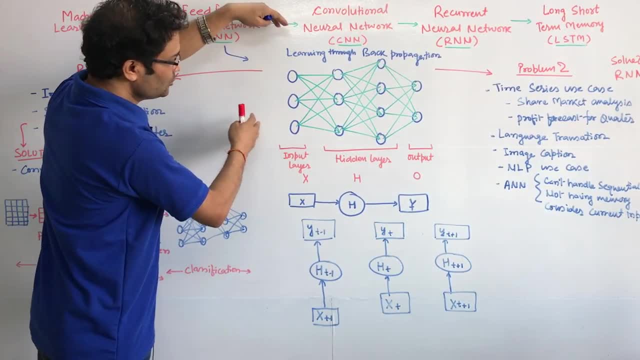 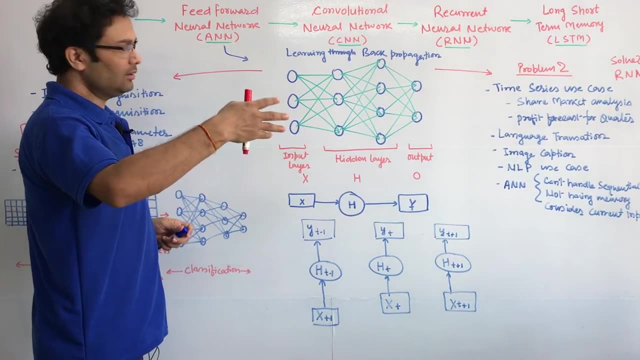 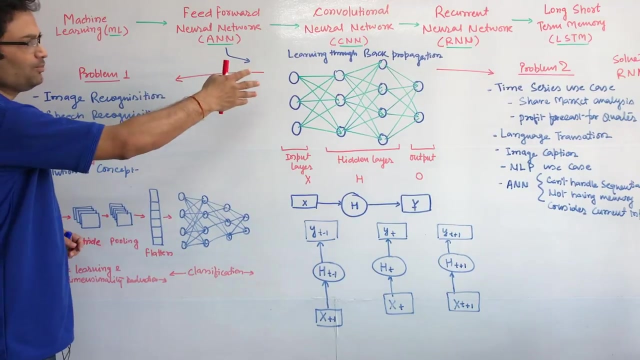 240 by 240 and if you give here input so number of input parameter is huge and the density become high and it will take the very good time and I cannot get the good performance and result might be not good If you use this kind of the input parameter with the ANN. 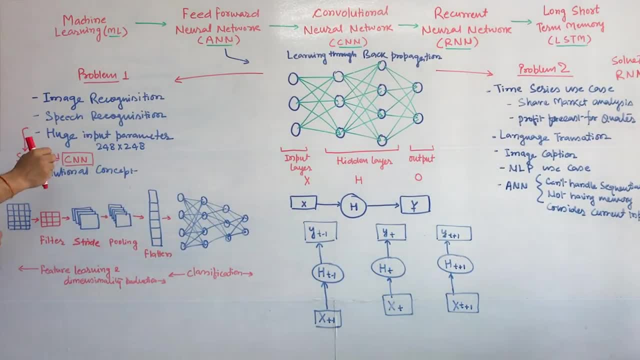 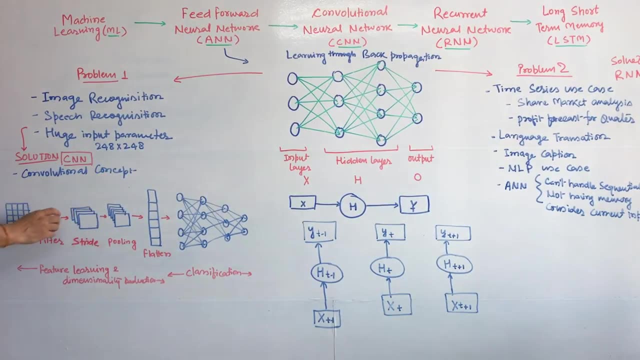 Okay, The solution is that we can use the CNN Convolutional Neural Network and the main concept is called the Convolutional Concept. Right? What would happen? You take one image. on that image, you take one small size of filter and move over there. 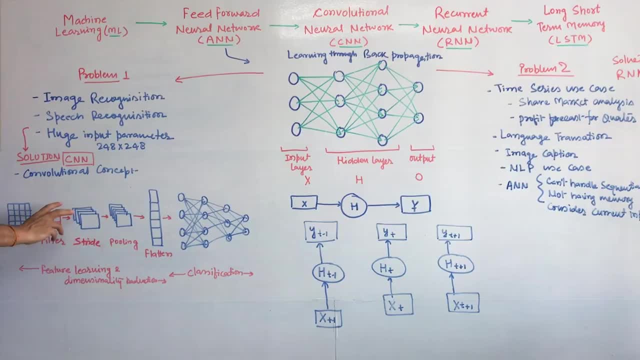 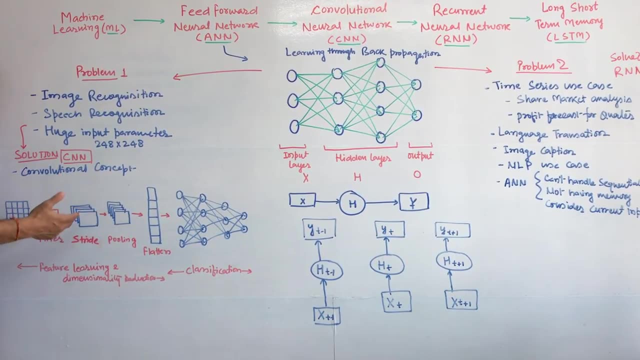 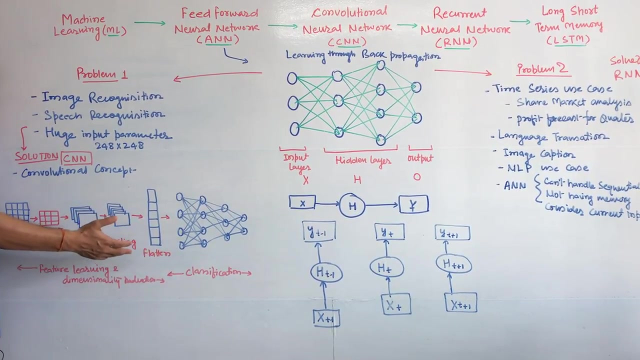 Right, One by one, one by one, move that, so it will reduce the dimensionality. having capture all the important features, then you can pass the different concepts, like the stripe pooling. in pooling we have the max pooling, average pooling, and then you use the threaten. 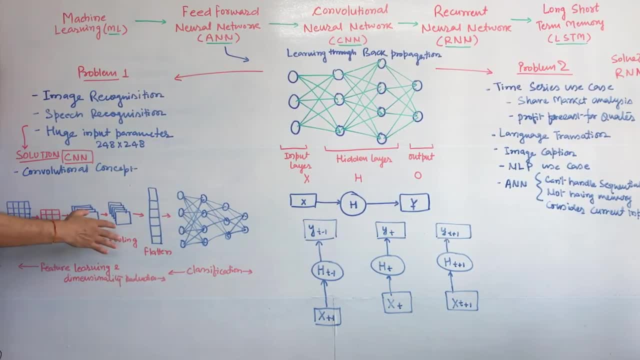 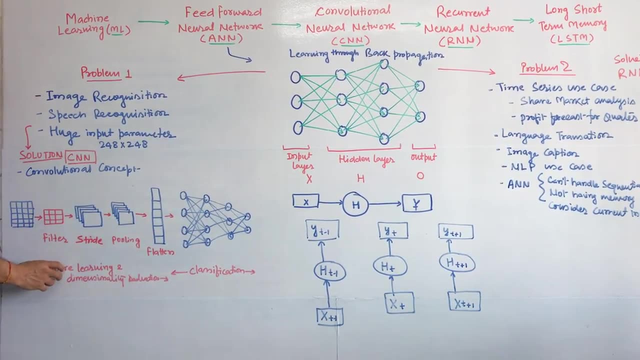 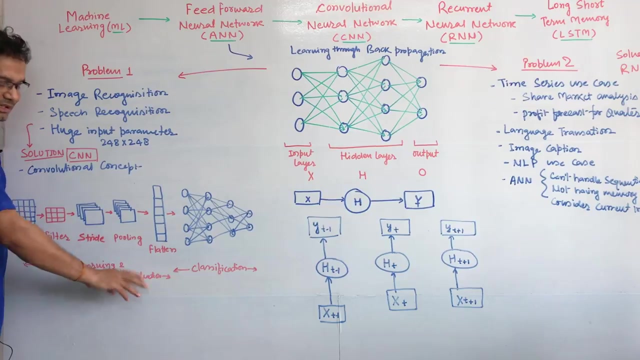 So I have already made one good video on this concept that we give the very good insight for the CNN. So what we do, from here to here, it will run the feature or the important feature, Preserve the important features. then there we do the dimension reductions, dimensionality. 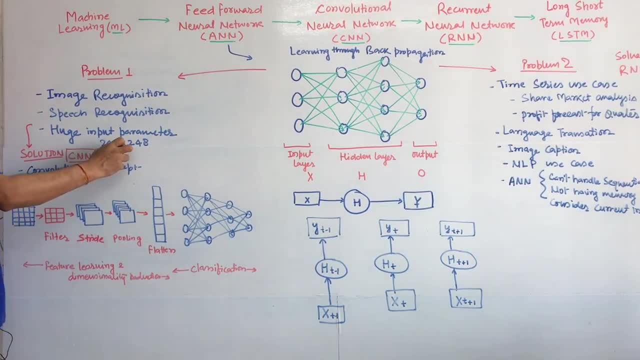 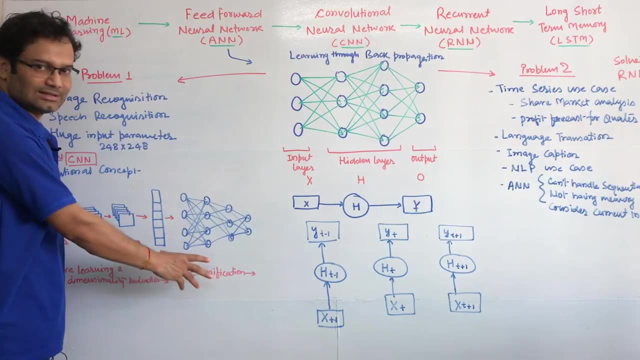 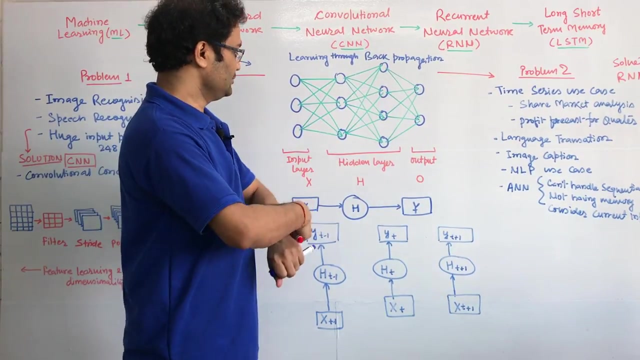 reductions. So there we reduce the size of this input and then we can pass those input again into the CNN kind of things and we will do the classification. So this CNN, we solve this problem. Now coming to the second problem of the ANN. So this ANN is work only for the one input. 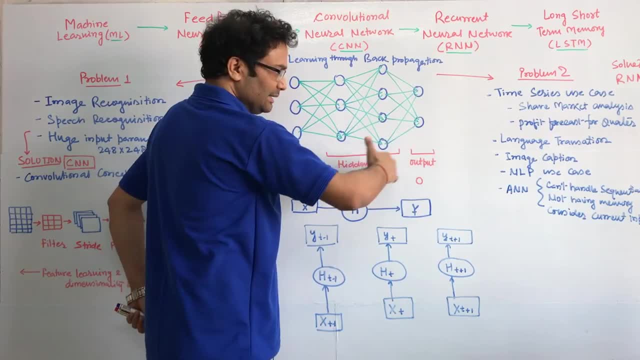 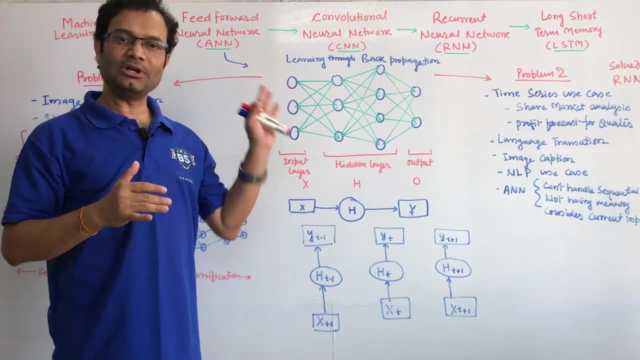 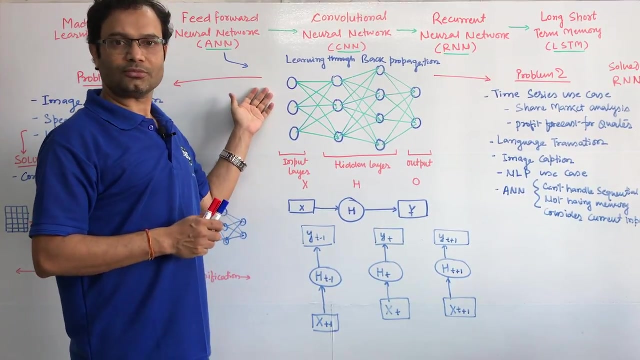 Means you give one input, You will get the output. Next time, if you give another input, it will give the output. but there is no any connection between the previous input output with the current input output, because it does not have any memory concept. 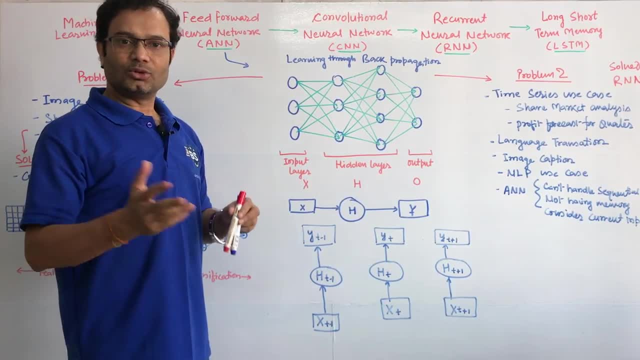 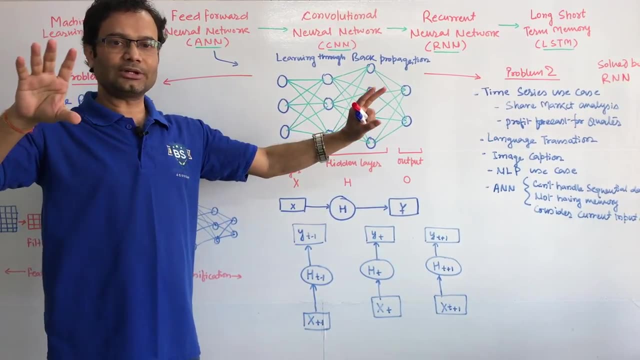 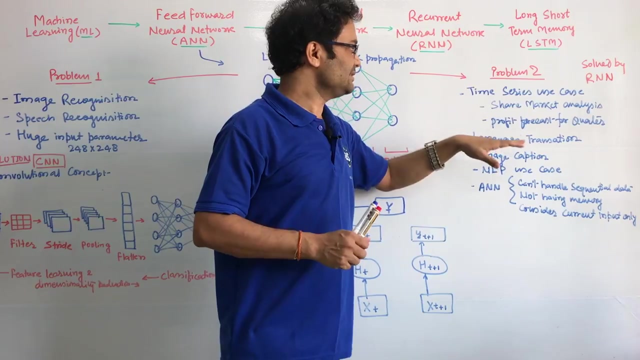 ANN cannot handle the sequential data, So take some use case like the time series use case. whether I have to analyze some data over period of time, We can't do that Right. That depends. It solves only for the one input, like the share market analysis or the profit forecast. 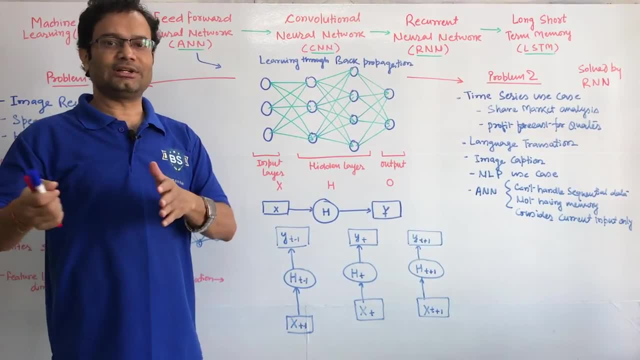 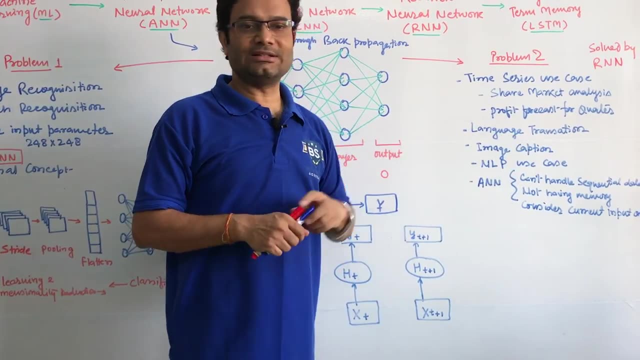 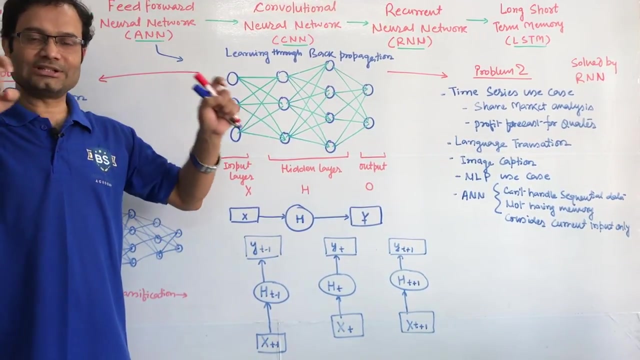 for the coming quarter. They need the sequential data and that use case is not good for the ANN Right. Take the example for the rank based translation. So if you sum translation from English to French right, So you have to give the complete sentence. 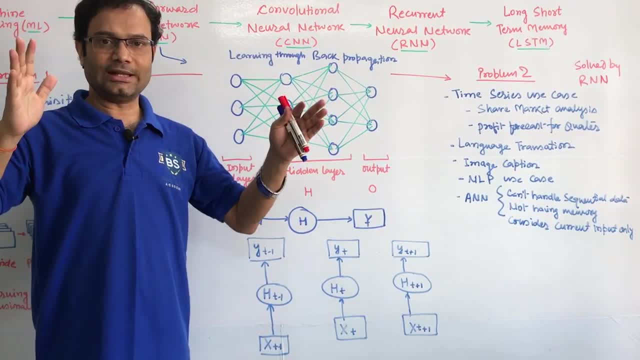 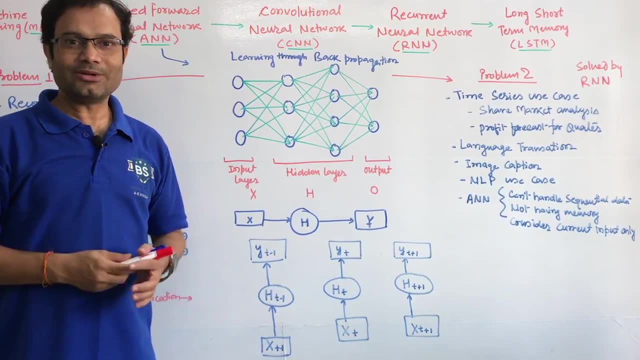 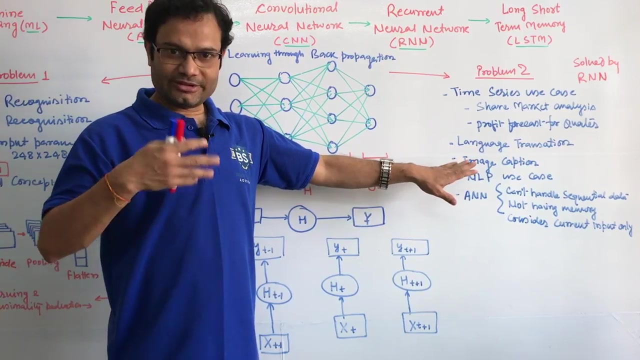 Input is not one. input is all the word of your sentence. then it will feed into the model and give the corresponding French word. It is not one to one mapping also. So one small example: if you say big cat in the English, if you translate in the French, 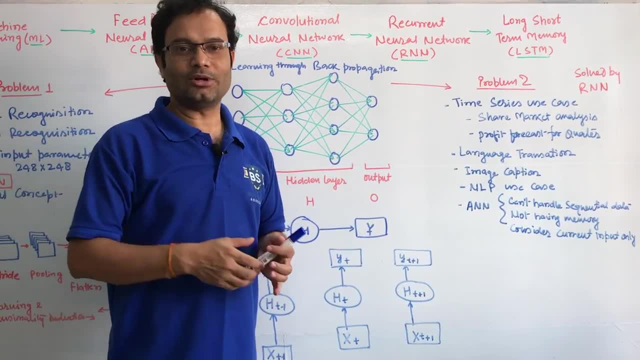 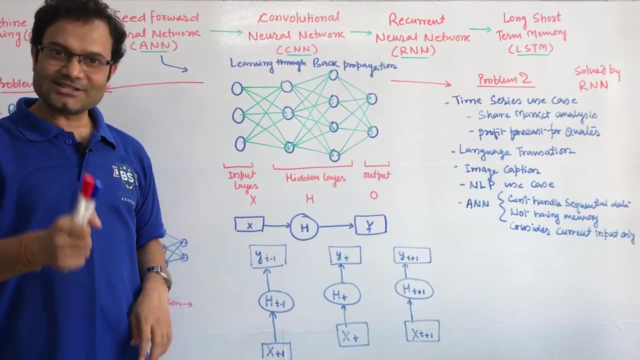 it become the cat big. So this is not one to one mapping. So those kind of memories, ANN does not have to solve this kind of problem And this is the point, we have to use the RNN. So all those things you are going to solve in the RNN. 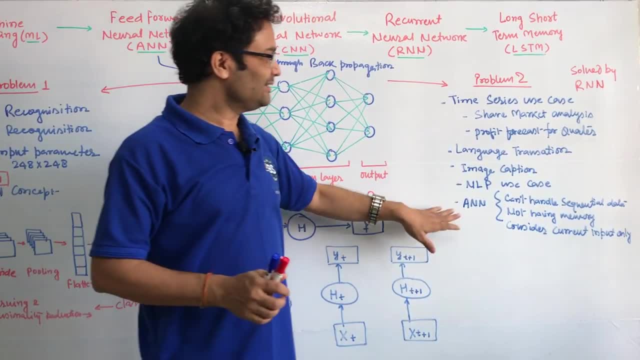 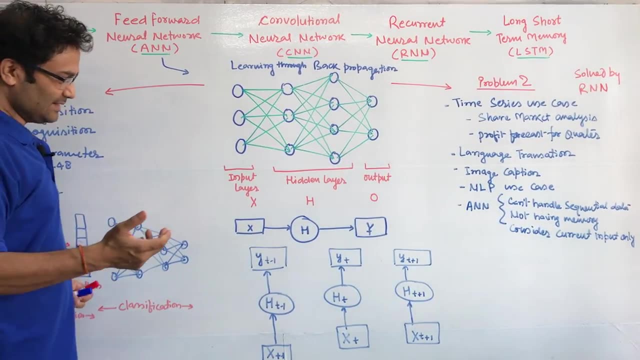 Now Let us see that, how you are going to solve the RNN and how to capture the memory. So idea is very simple, not very complicated, just I need your some attention. So what I explained in the ANN, this is input layer, hidden layer, output layer. 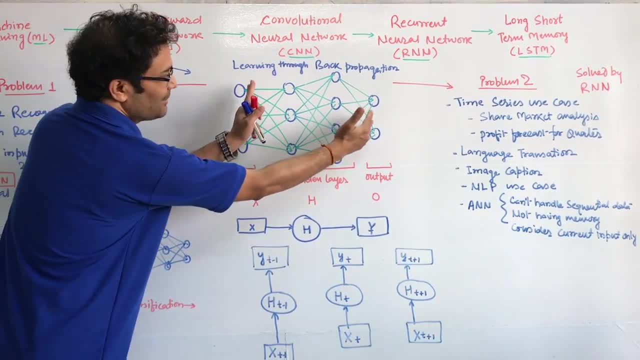 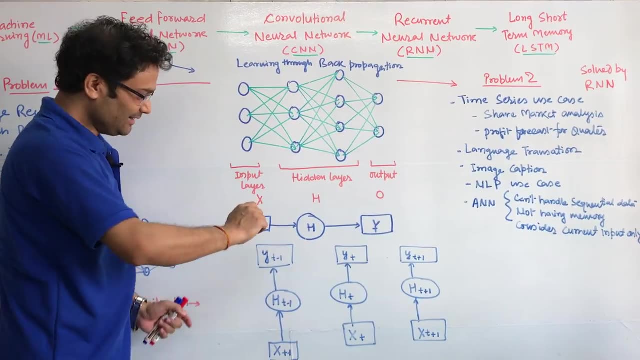 So this is the. for the simplicity, you correct all those things in this hidden that could have the multiple right. And just for understanding the RNN, just you prep this side right, just so. take this one and keep like this. 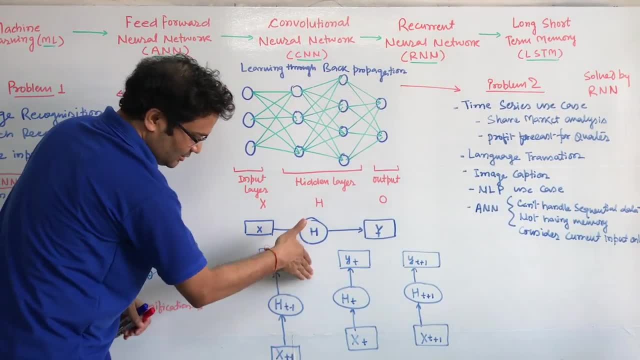 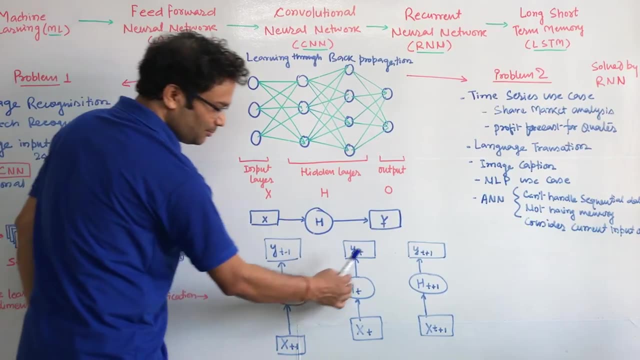 So Y is came here H and X. So this is the ANN right. This part is the ANN. this part is the ANN. So we have to use the multiple ANN to solve the sequential problem. So we can take the multiple ANN. 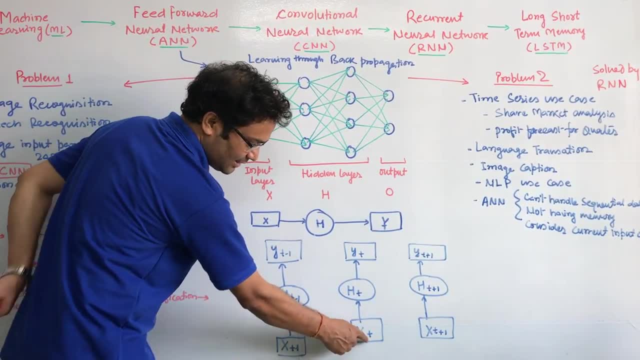 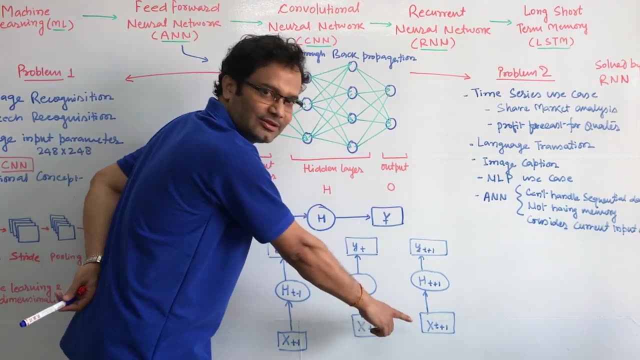 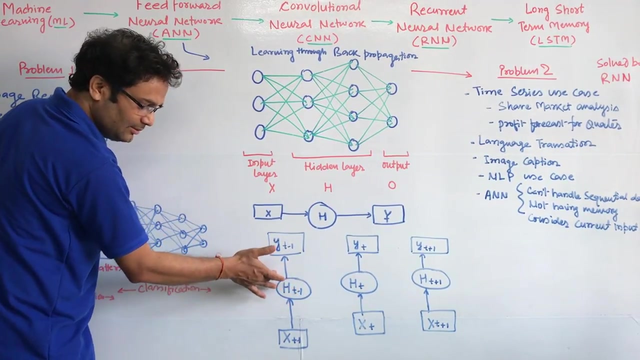 And if you see, this is a time series, So this input is at the time t, this previous input at the time t minus 1, next is the t plus 1.. Right, If we take the t minus 1 input, if we go the hidden layer for the t minus 1, it will give. 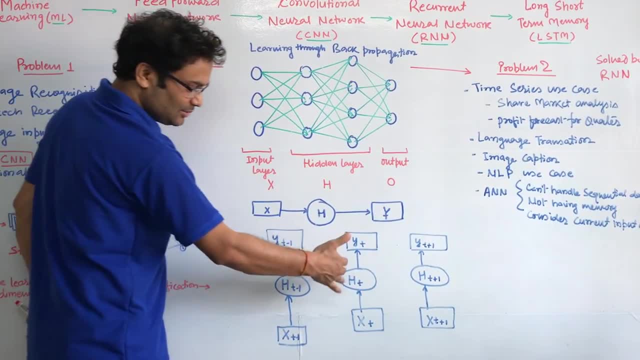 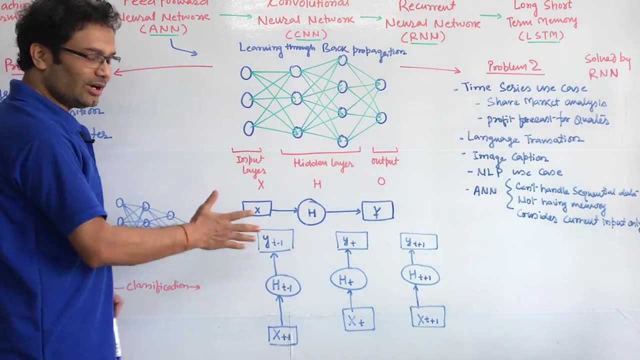 the output Y at the t minus 1.. The same thing, this output at the time t. this output is the time t plus 1.. But question is that how we are going to preserve the memory? What is the output for that? how it is going to pass. 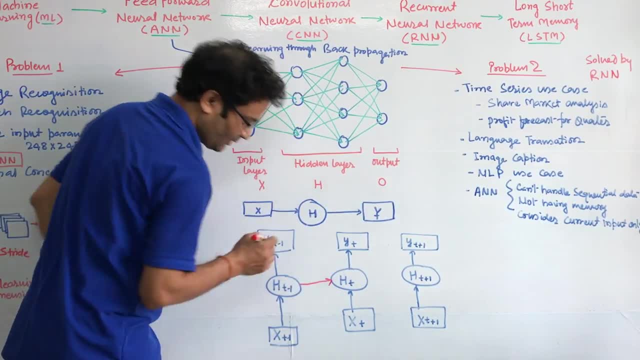 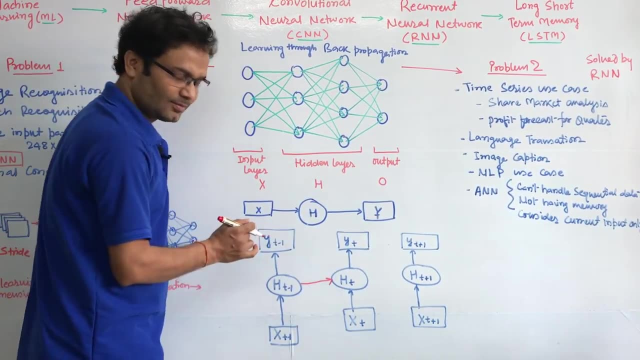 That magic line is this. So what I will do: when this hidden layer will give the output to Y, it will give the output to Y. It will also pass the same output to the. this ANN layer, right, this will pass to this. 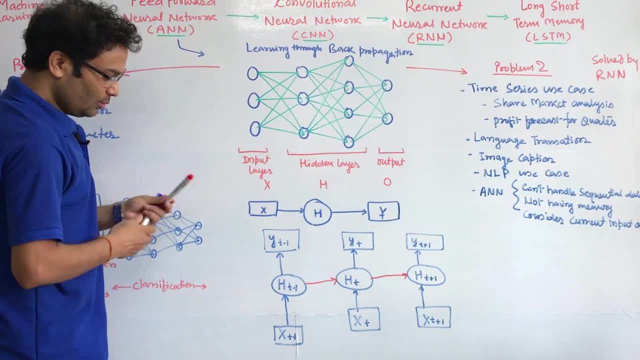 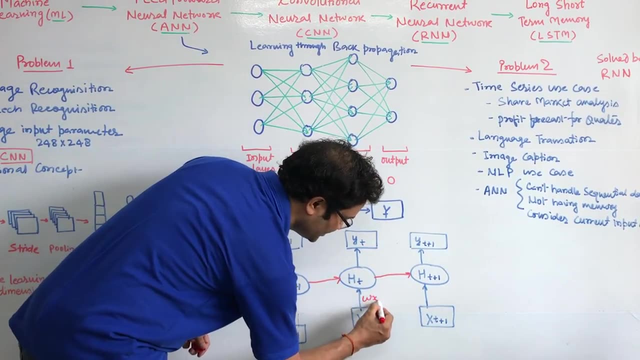 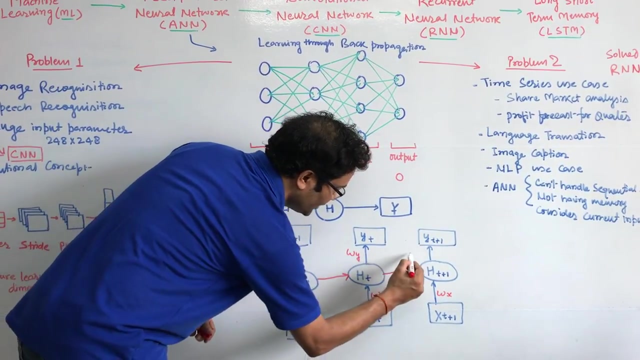 one right And you know we have some weight here. we will have some kind of weight, If you see, the Wx, Wx, Wx, right, And we will have here Wy weight, Wy weight, and we have the Wy weight. 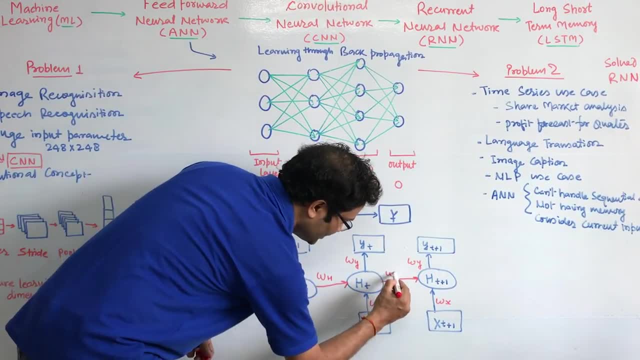 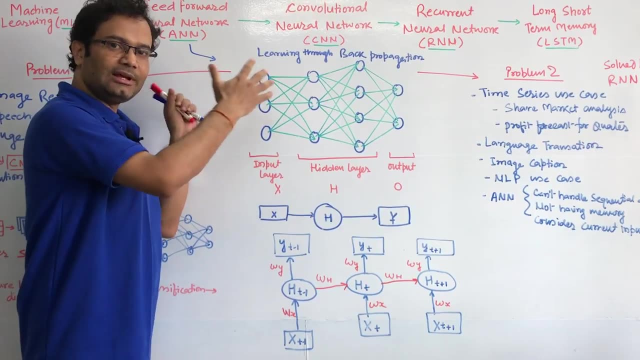 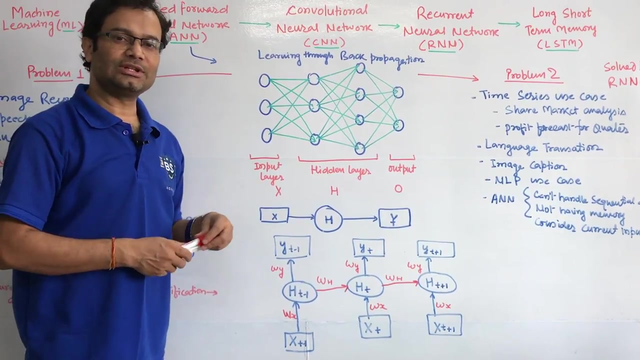 And this nu is going to Wh weight and W weight Right, And this is the main fundamental concept of the RNN. So let us take the bigger picture and we try to understand how many different kind of RNN we have to solve the different kind of use case and what is the mathematics behind. 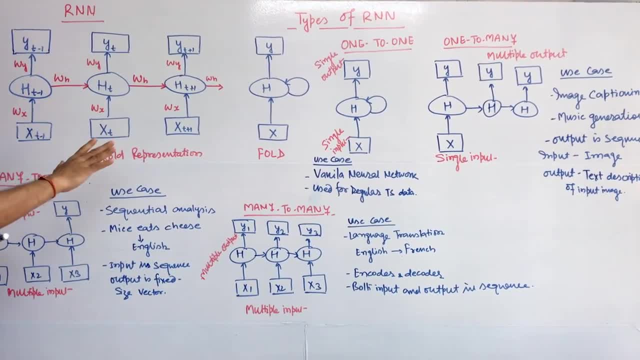 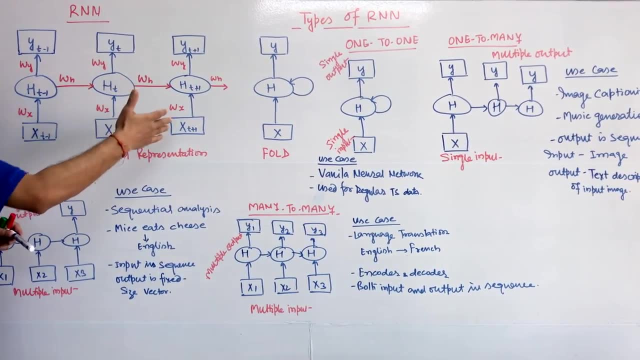 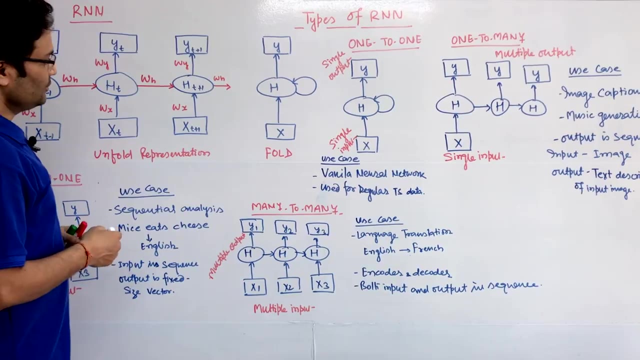 that Image here And this is a traditional, typical recurrent neural network diagram. So this is the way we represent the RNN and we have the multiple intermediaries And this is called unfold representation. everything is unfold. To make the easy representation, whatever is to do, we make the fold everything. 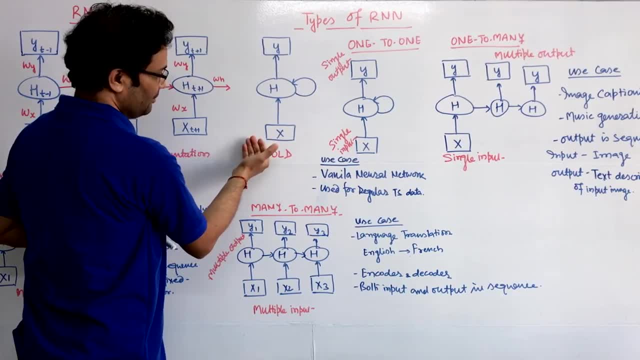 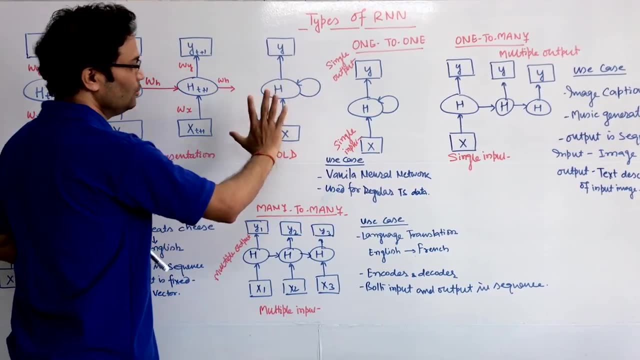 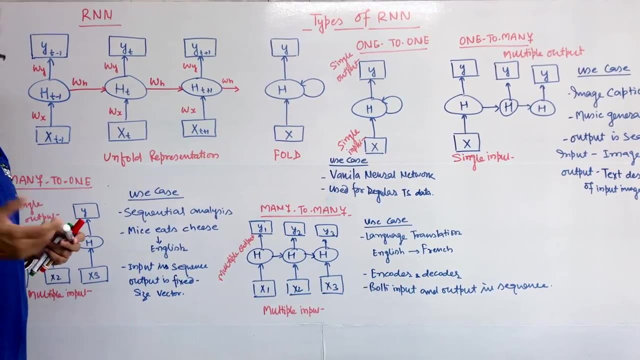 collapse and showing in one diagram and many input, output and the recurrence recurrent, this layer, right? So this is the way we can show this, the fold way of representation. this is the unfold representation and this is called the one layer, RNN, right, If you? 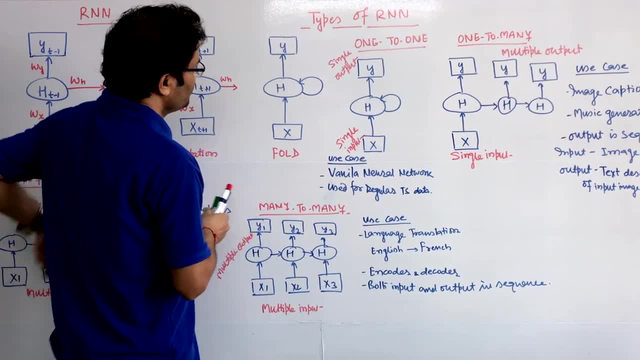 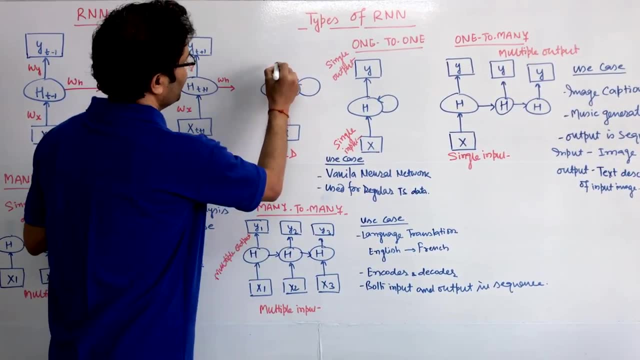 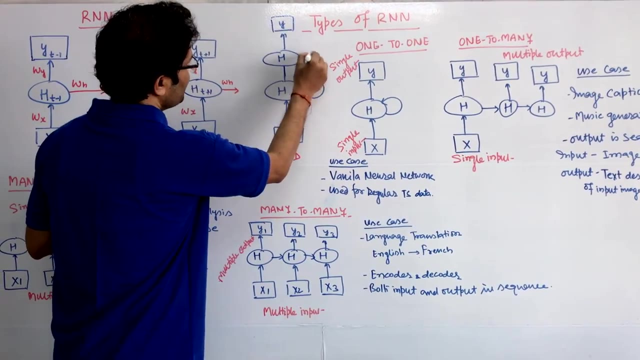 want to make the multiple RNN. so what you have to do, You can do that- you can make one more layer of the hidden layers, right? So we can make the one more and then become the output here. So we can say: this is the multiple RNN. ok, multiple RNN. 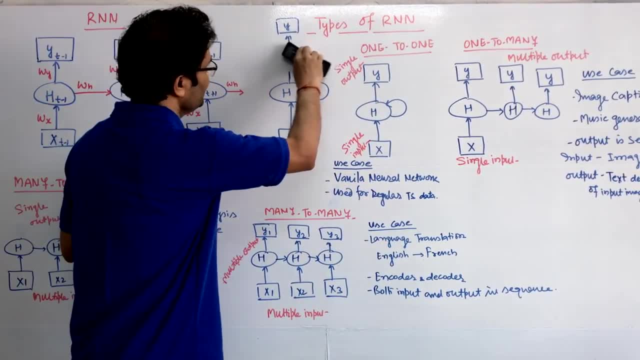 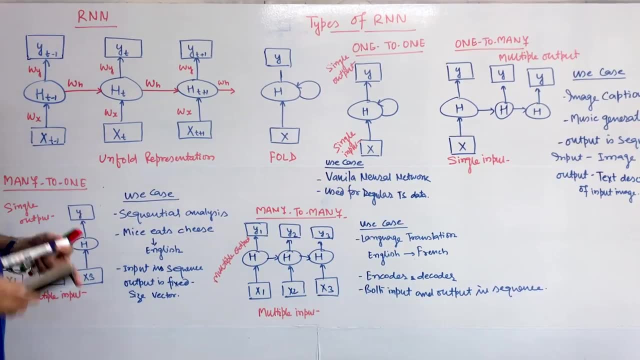 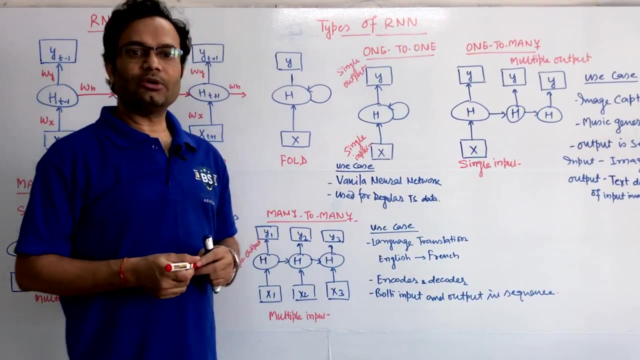 But for the easy representation or the easy understanding, let me just keep the, let me use the sample. So this is the single layer RNN. right, So now we have a different kind of RNN. So one to one, one to many, I am going to explain one by one, with the use case, what is the? 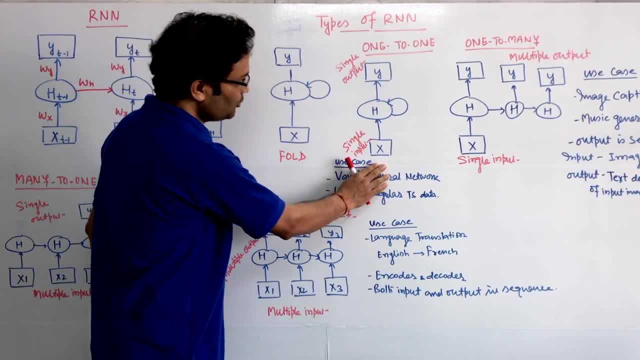 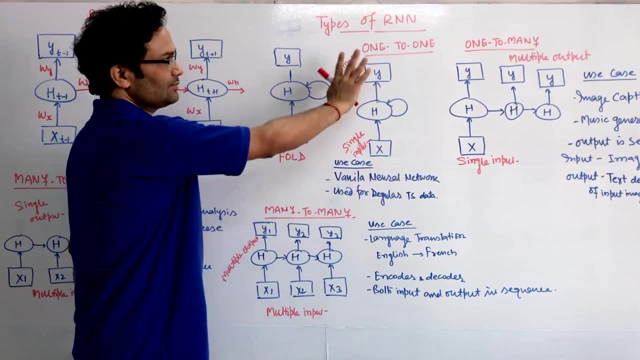 use case If you take the single one to one. so single input and a single output and they have the multiple hidden layers, but we can represent in this way. So what is the use case for the one to one RNN? This is called the Benira neural network train, very traditional. 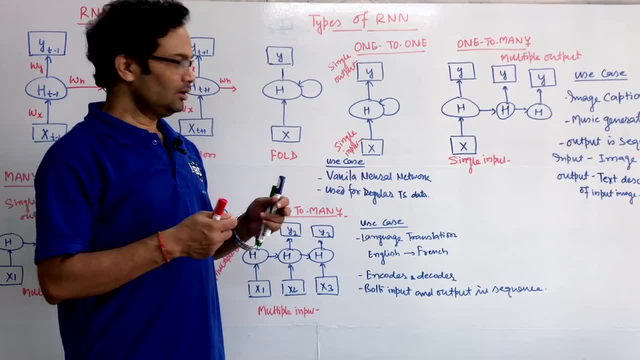 RNN And if you have any training then you can use it. So what is the use case for the one to one RNN- This is called the Benira neural network train, very traditional RNN, and if you have any time series, so one single input time series to get the output time series, then this is: 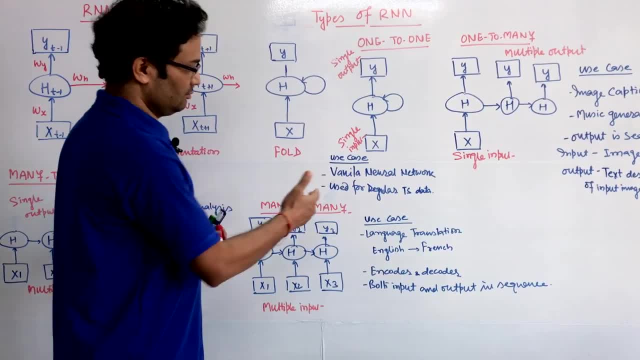 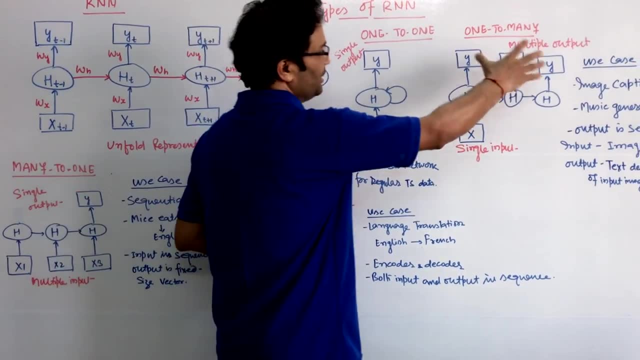 the way we can use that right. This is a single or not the time series, the actual machine learning, where you have the input, single input and single output, right, And then the one to many. we have the single input but we have the multiple output. So 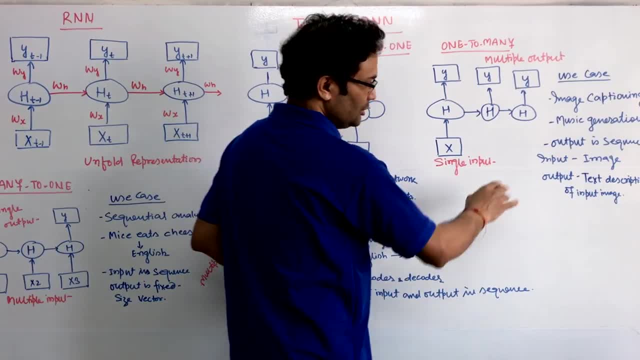 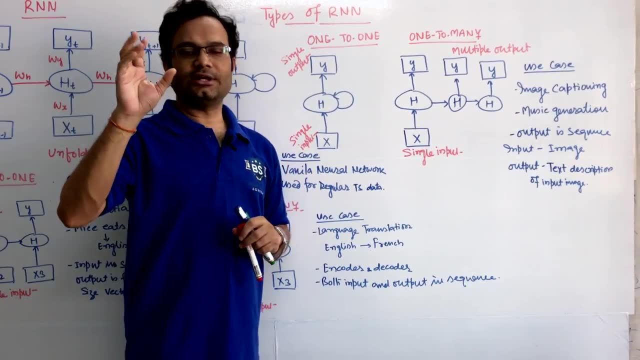 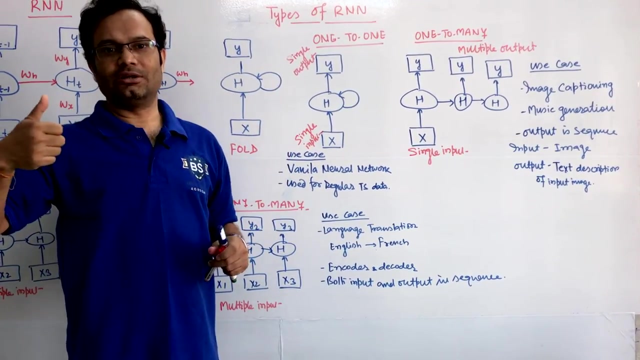 use case: see the image captioning. So input is the one image and output is the test description of the image. See if I saw one image that one boy is studying with the book, right? So image is one, but the captioning is big. one boy is studying with books, right? So 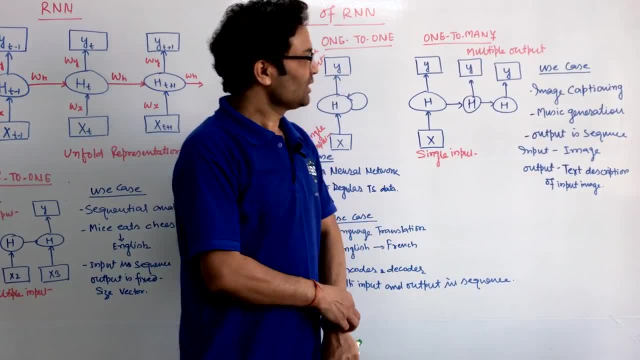 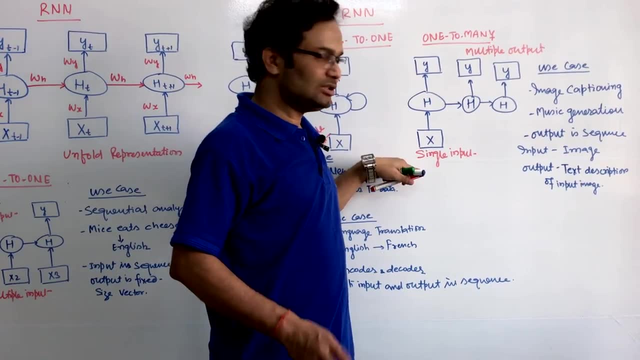 output is the test description of the image right, And that music generation is also there. So you can see, output is the sequence. the sequence is here, but the input is the single unit. right Now it is study. take the many to one in. 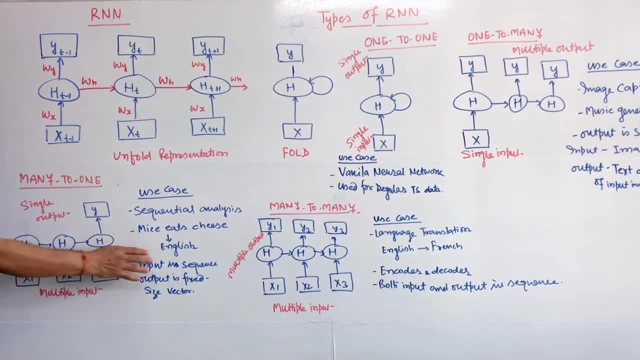 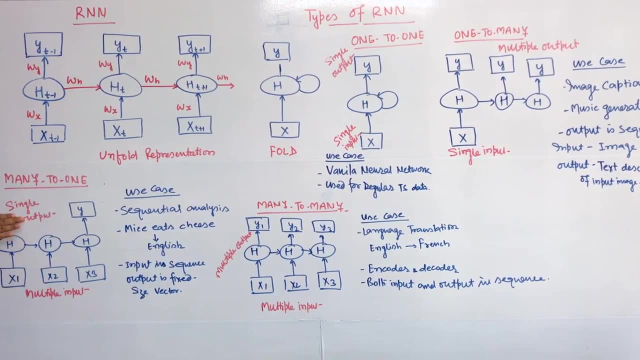 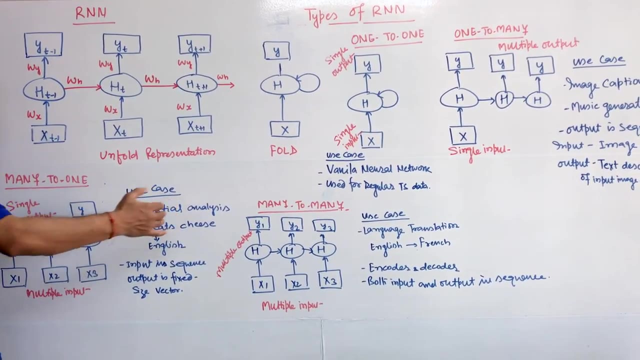 In this we have the many input means, input in sequence and output is the fixed size vector. So multiple input and the single output with the multiple intermediate hidden layers. So the main use case of the sequential analysis means if you have the data in the one sequence. 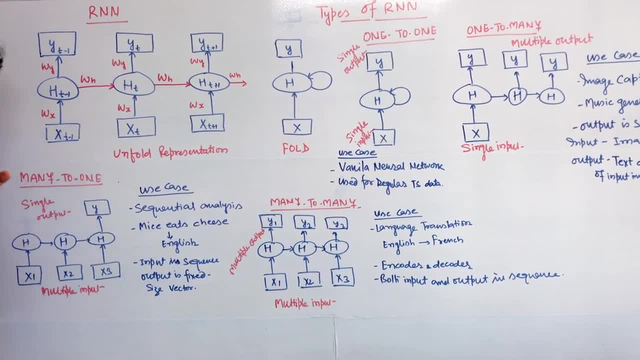 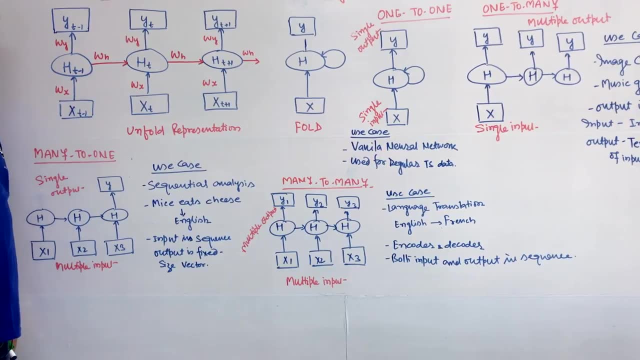 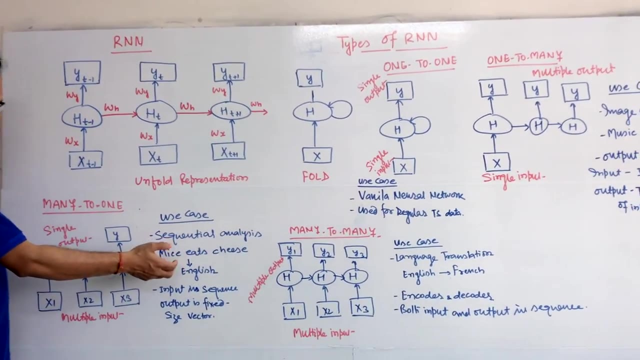 and you want to one output, that time you can use Very easy. or the, that common example for this many to one. If you give some sentence in the Google, they will tell you which language is this. Suppose if I say that one mice eats cheese, so he can say this is the English sentence. 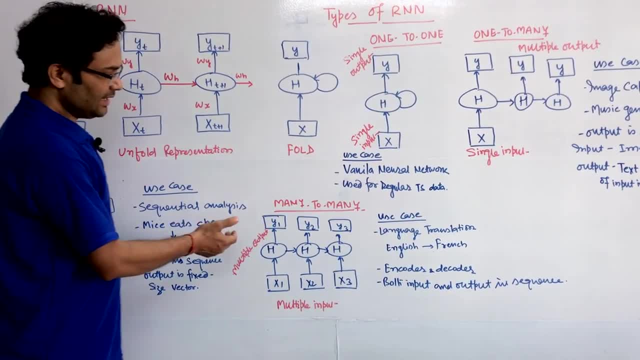 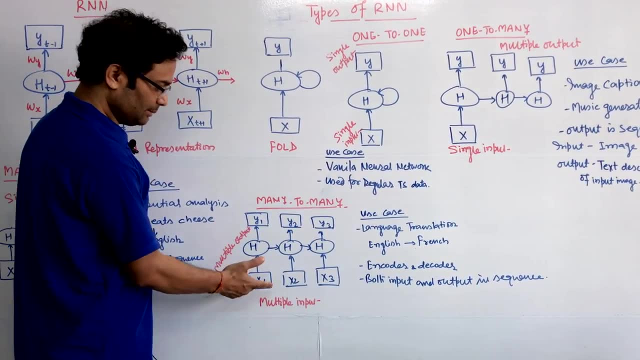 This kind of use case you can do for the many to one. many is. the next is the many to many, where you have the multiple input and the multiple output. It is not necessary that if I have the three input, output is also three. no, 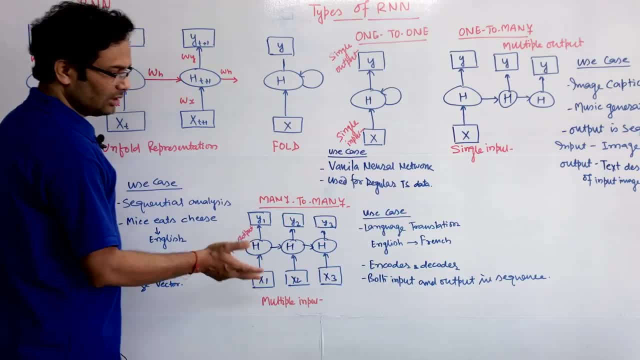 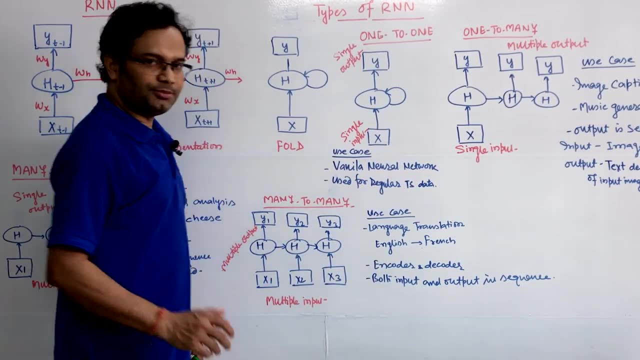 That the number could be changed depend upon the use case. So what is the use case Use, main use case for many, to many, is the language translation. So if you translate something from English to French, so as I already told you that the 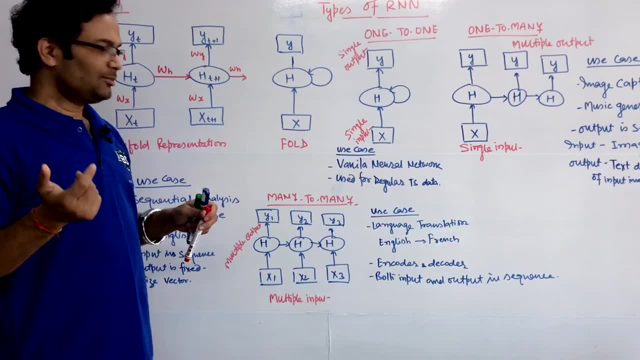 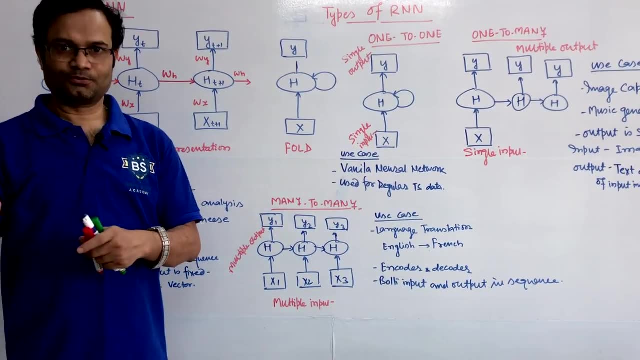 number of word is not exact: mapping. One example I said: if you say the big cat in English, if you translate in the French you become the cat big. So this kind of things you can use the many to many, and you can also use for the encoder. 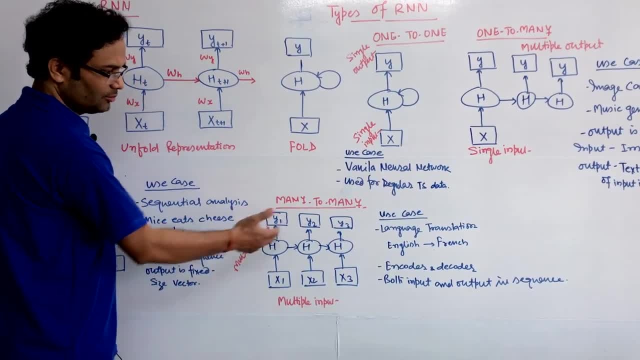 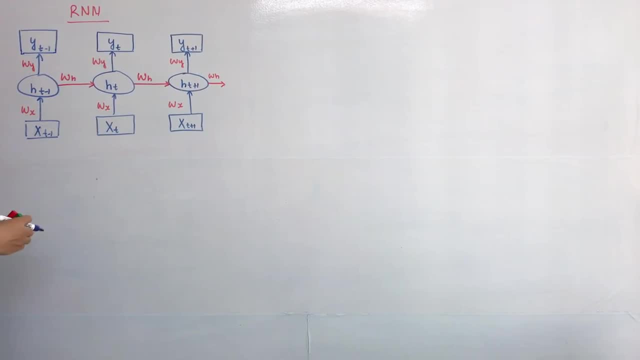 or decoder And both here you can see. So you can see input and output. both are in the sequence. Let us discuss the math behind that, how it is going to calculate and how it is going to that initializing the weight and that the update the weight. 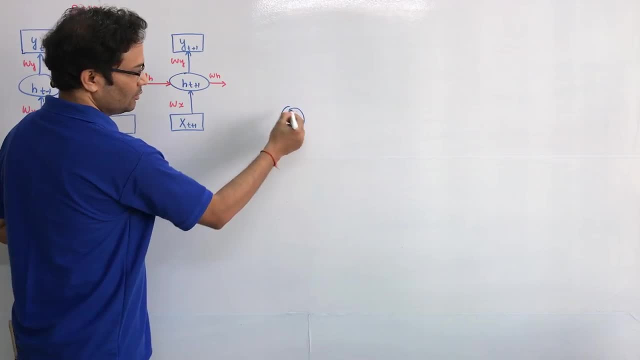 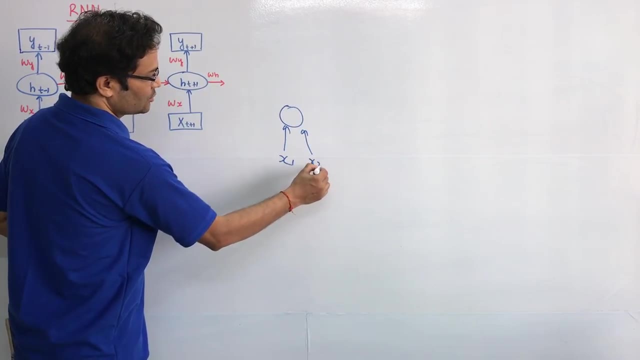 So, as we know already, if you take the one perceptron- we have already studied that and suppose we have the two input, x1 and the x2, and then we have to go one output and we have the one bias. So how is to do? and we have the weight w1, w2.. 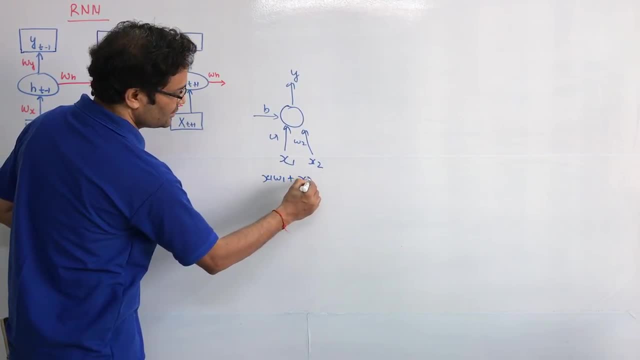 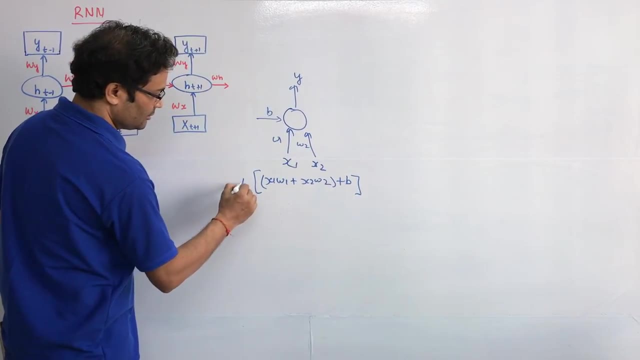 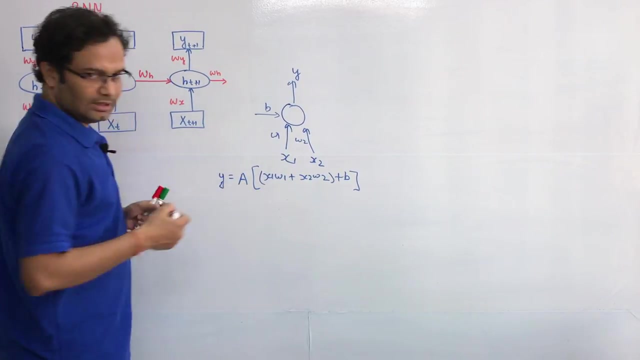 So we used to do- we have already studied this one- and then first pass the p and we pass everything through the sum activation method and that is the result for the this y, y. The same way what we have studied in the feed forward network. we will do the same thing. 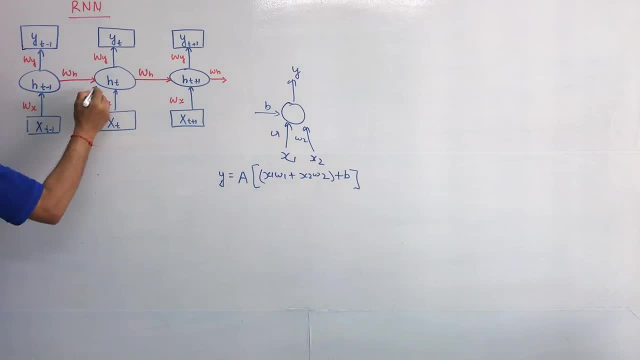 So if I want to say what is the feed forward network, So if I want to say what is the feed forward network, So if I want to say what is the feed forward network, So if I want to say what is the output for this? 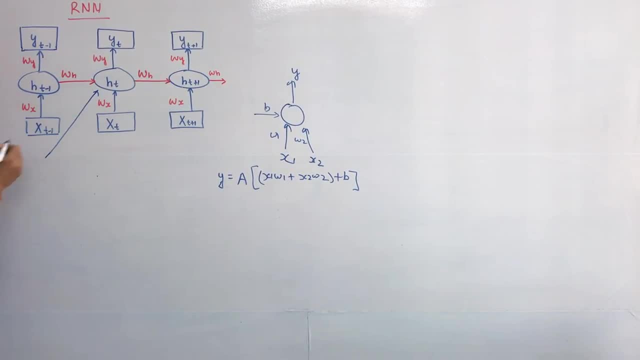 So if you want to calculate this output, so let me first what things is going to the activation. So just if I use the, this is for the hatch hatch. So if you see the hatch at the time of t, what will happen? 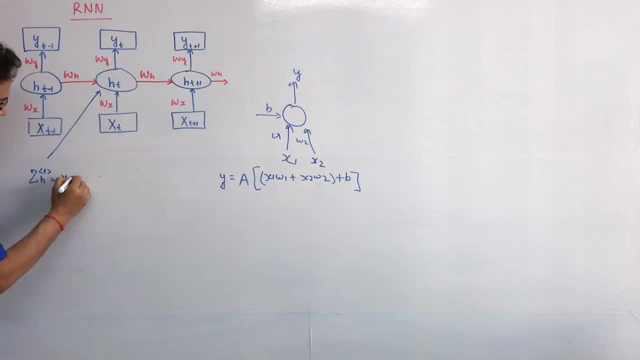 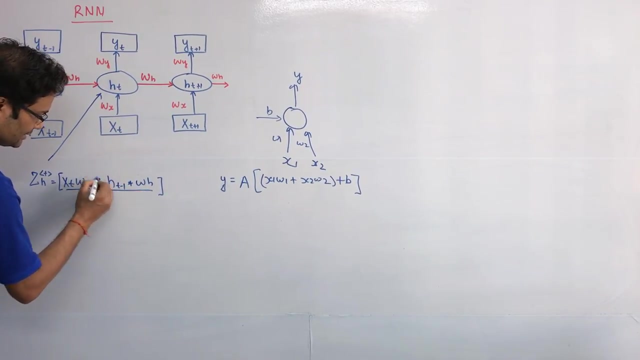 This x, t right plus into wx, the same way what I did here and here: this hatch is going to be t minus 1- into this weight w hatch, weight right, and then, and this, this is total, this, multiply this. this multiply this addition, this, and this is the bias, right bias for this. 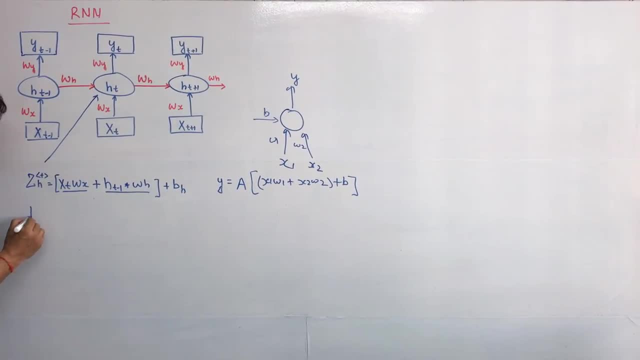 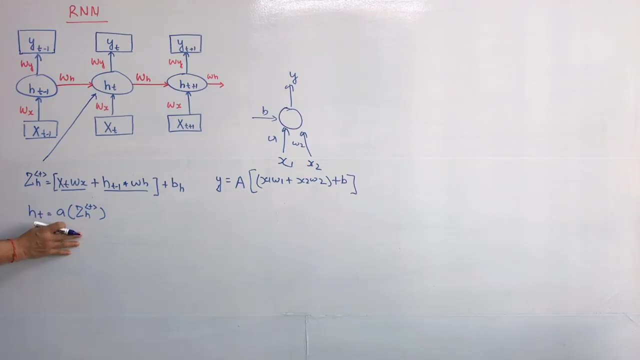 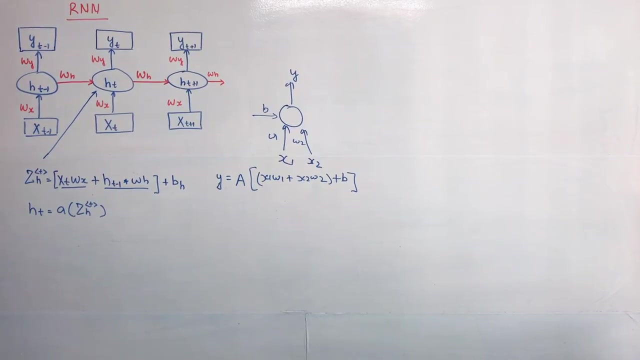 one, and this will go to the activation. then we can get the h t, So this will go to the. so this is the output, for this is the value for the h t, right? the same way, if I want to get the for this output, this y t, what is the value of y t? 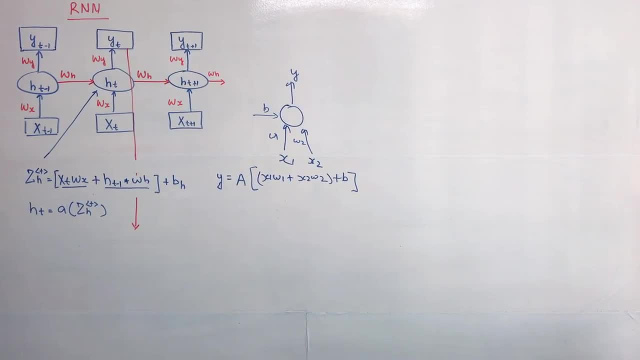 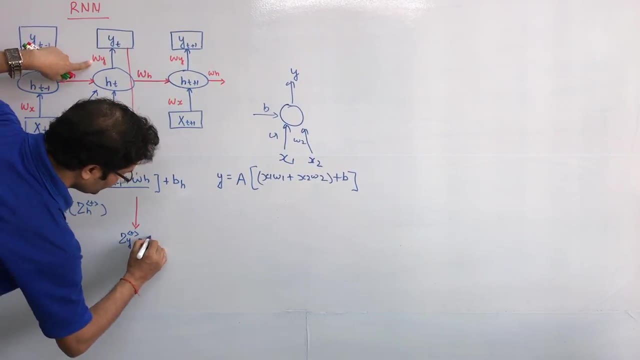 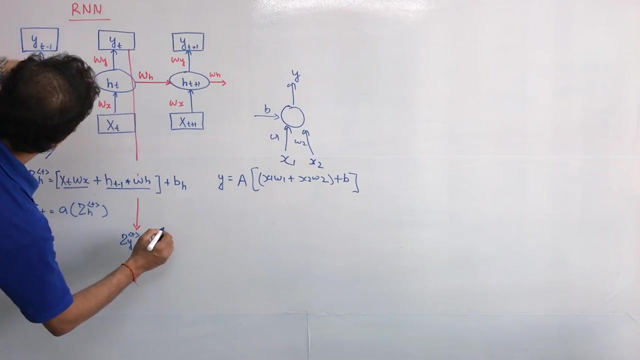 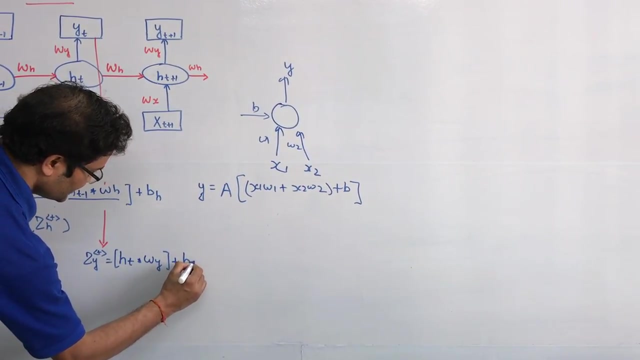 So let me put it here. So again, if we calculate the z y at time t, so this time w y or this the h t, that we have already calculated h t into this w, weight for y and bias for this the y and 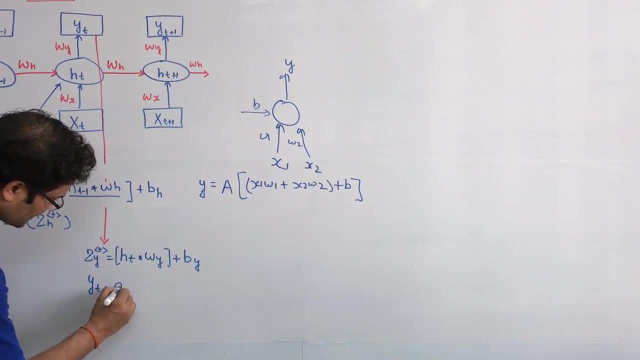 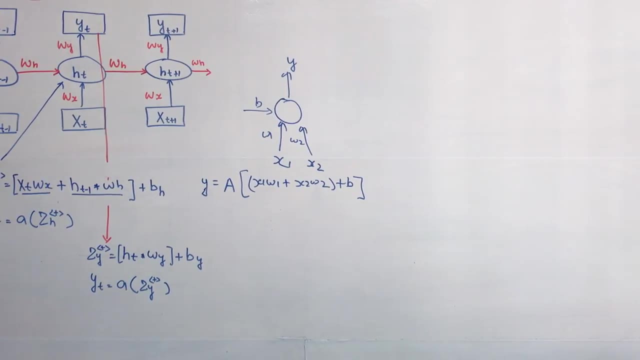 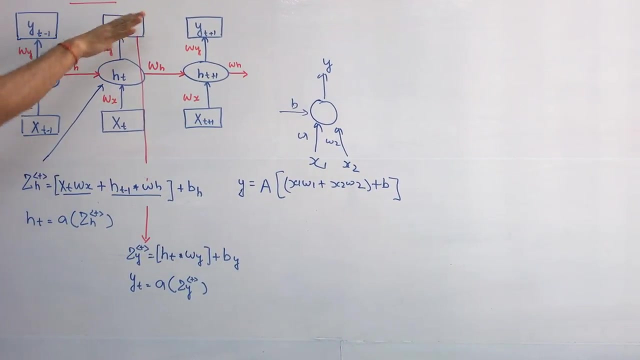 the value of y t. again, we pass some activation method, this z y t right, how? this is the mathematics, this is how it is going to calculate inside the RNN. So once we get the y multiple, y multiple output right, so we have the sum, the differentiate. 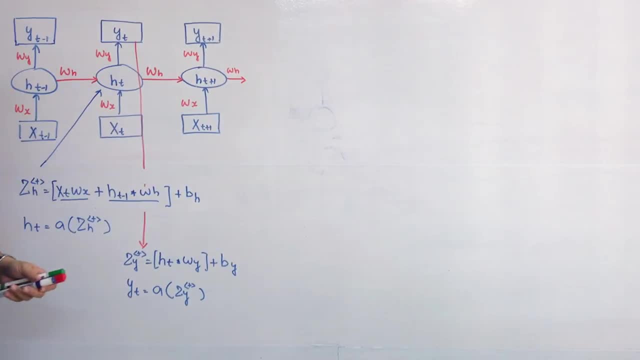 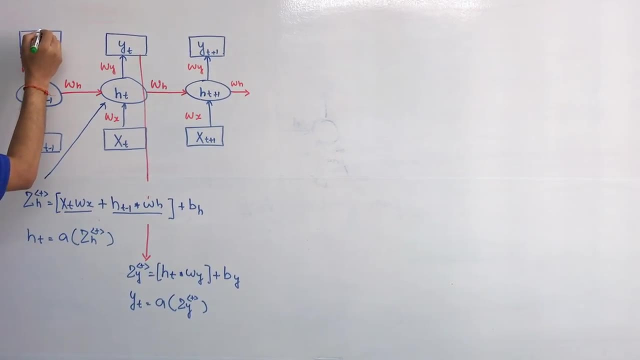 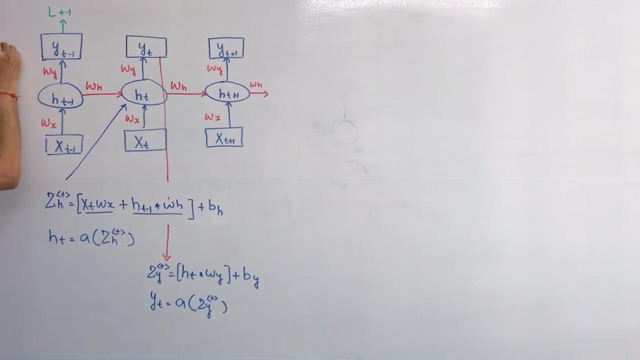 we have to find out the errors between the actual y and that the model's y right. So if I say this is the, if I want to say this is the loss. loss for the t1,. loss means the difference between the y, t minus 1 and t minus 1.. 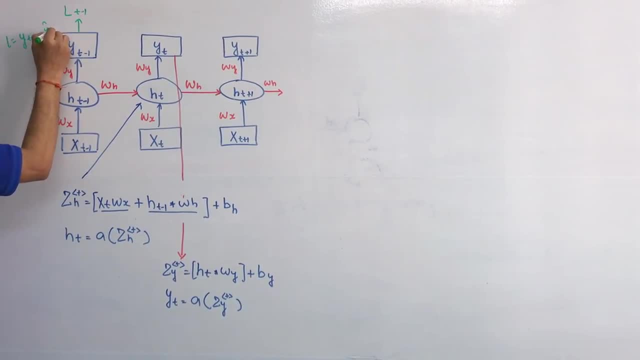 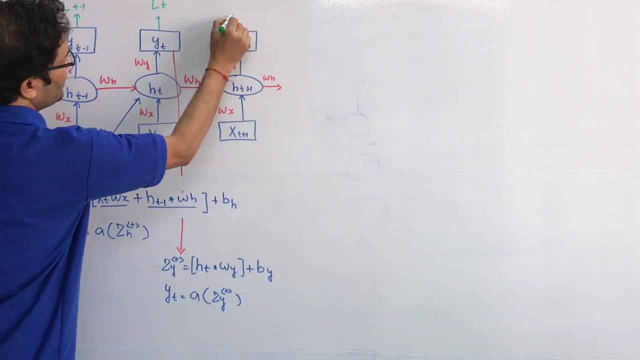 So if I say this is the y t minus 1 and with the model t minus 1, right, we have already know that. and for this output, if this is the loss t, and here this is the loss t minus 1.. So now what we do. 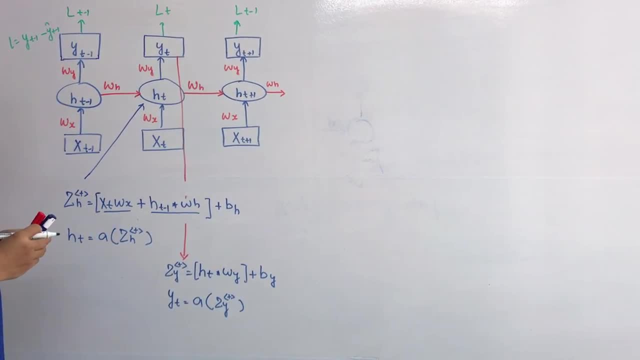 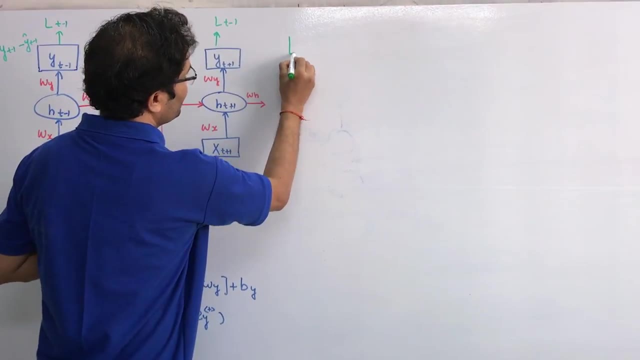 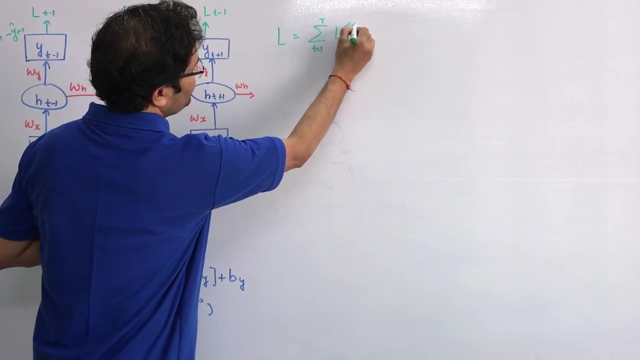 We have to do the back part calculations how we used to do. We use the gradient descent for that. we have to calculate all the loss. so we take the total loss summation p, So p is equal to 1, it will go to t. it will calculate all the loss, right. 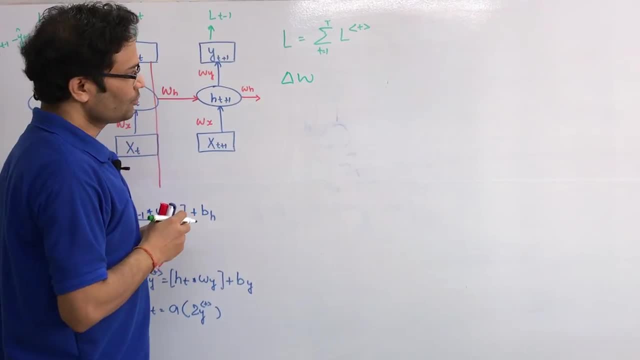 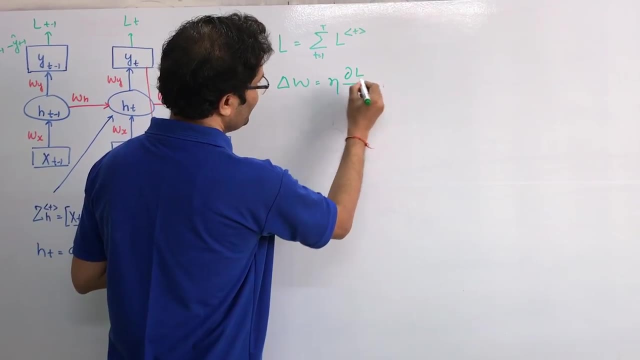 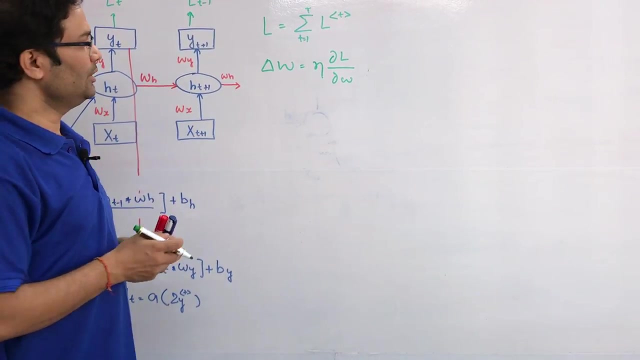 We have to find out the change in the weight. so what we will do, We put the learning rate and whatever the errors we got it and by the weight right. So this is the change rate of the error with respect to the sum weight and we find out. 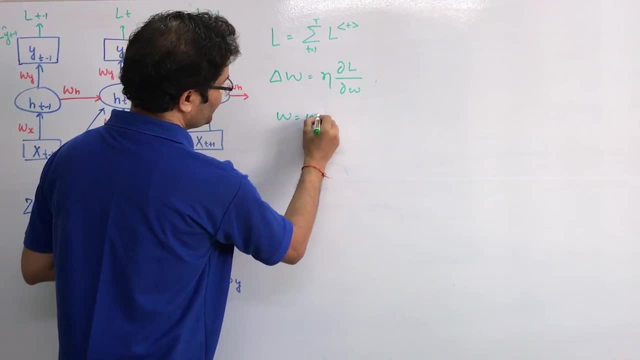 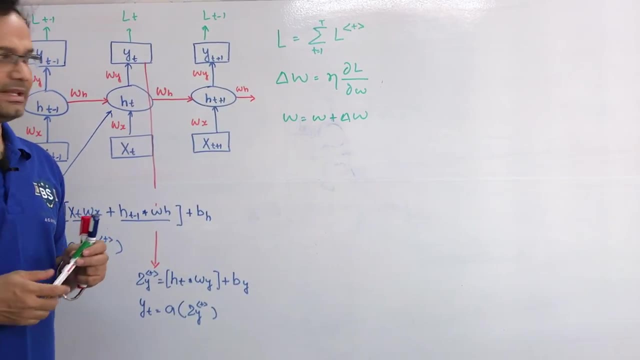 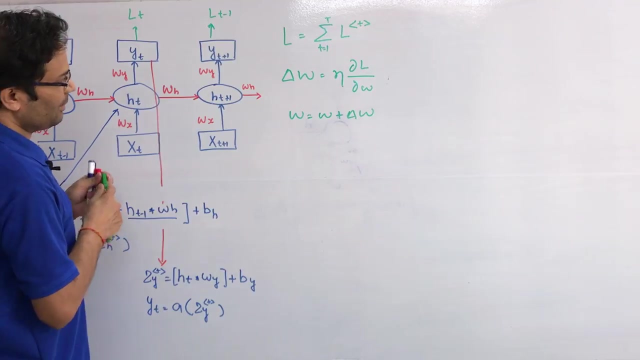 and then we update the weight with the function. So this is the way we modified the weight to find out the minimize the errors, right. So if you see this how it will happen for the each weight, it will update, right. So for this it will come here, it will do the back, back part progressions, so it will 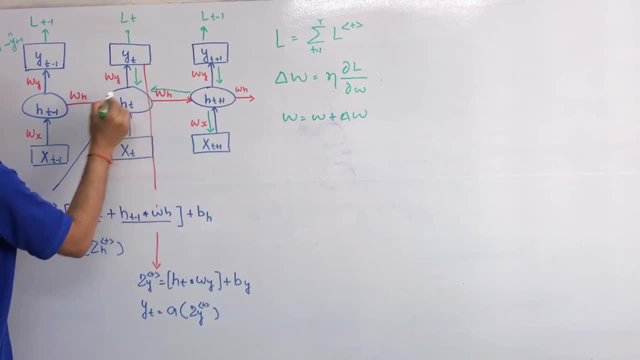 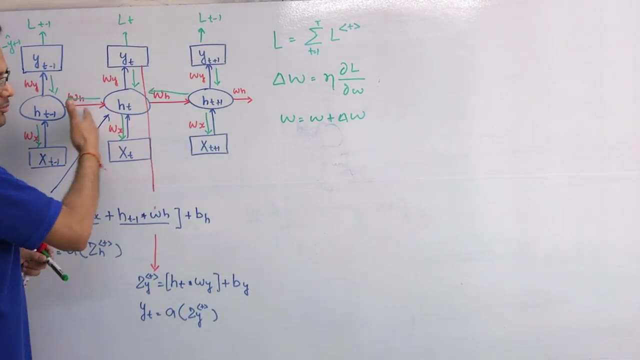 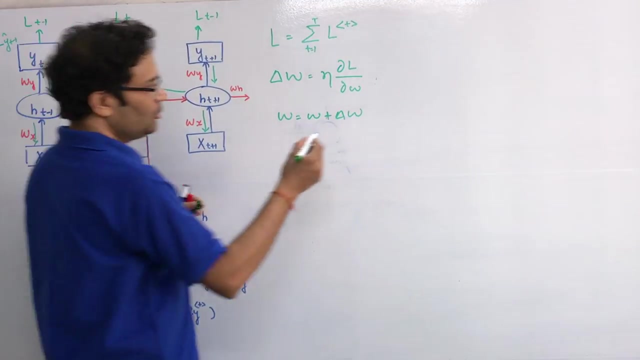 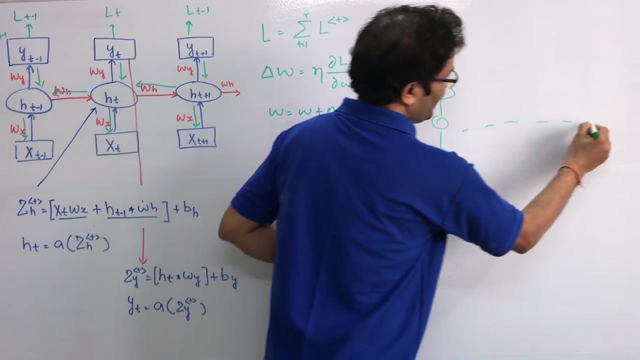 do like this. right, It will update all the weights, right? This is the way it do. the backward progressions Now you think is that, if this is, the number of this intermediate layer is huge. so suppose, if you have the one layers this way and up to 100, you have the 100. 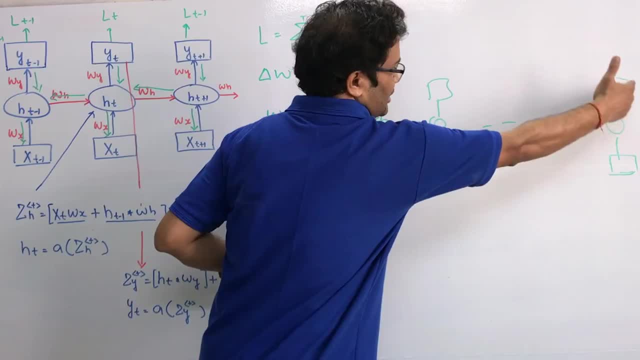 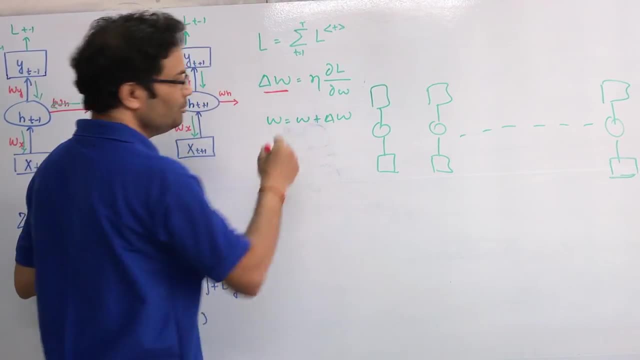 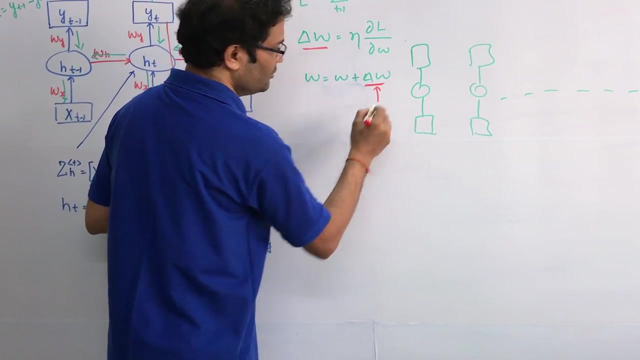 So what backward progressions will happen? it will come, it will start from here to go here, here, here, right, And at every step, that this rate we going to minimize, minimize, minimize. Once upon the time, you will see that the, this value is the very negligible, very near to. 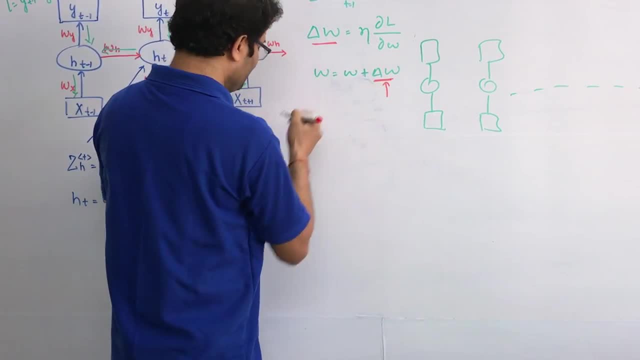 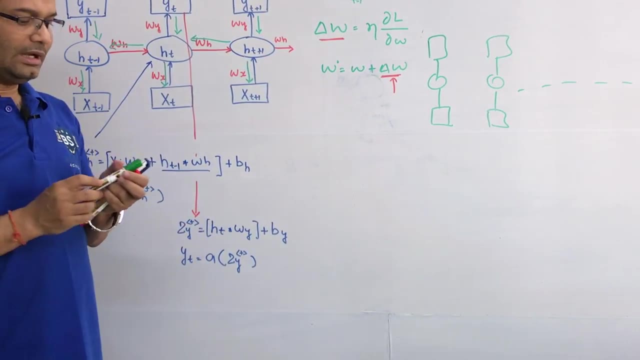 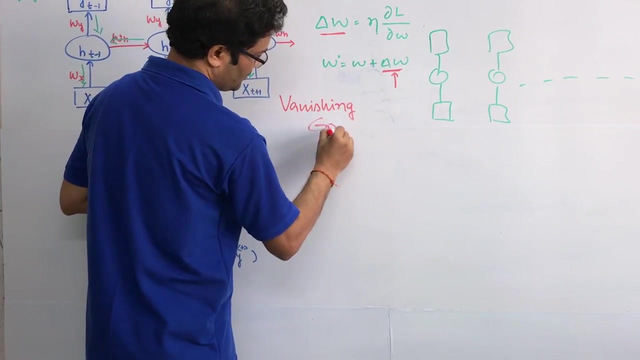 the 0 right and in that condition there would not be any change in the weight right. There is no change in the new weight, So in that way it will not work and that problem is called the vanishing error- Gradient problems.